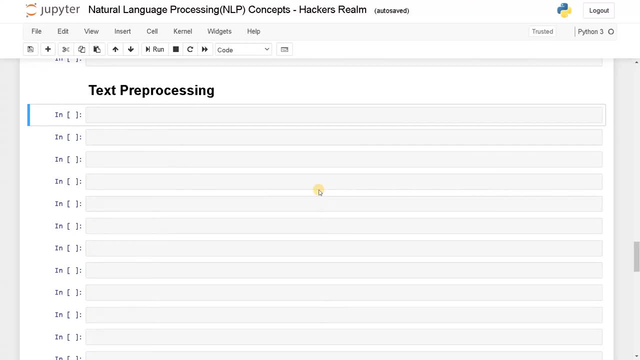 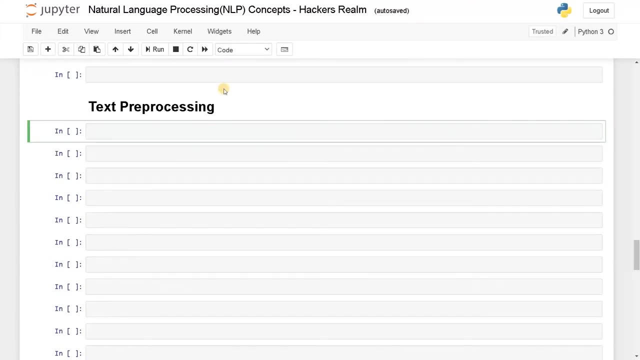 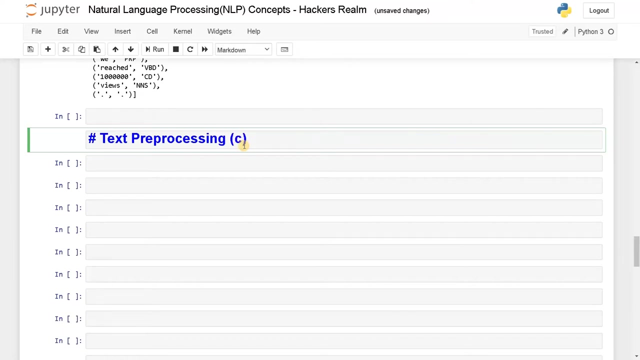 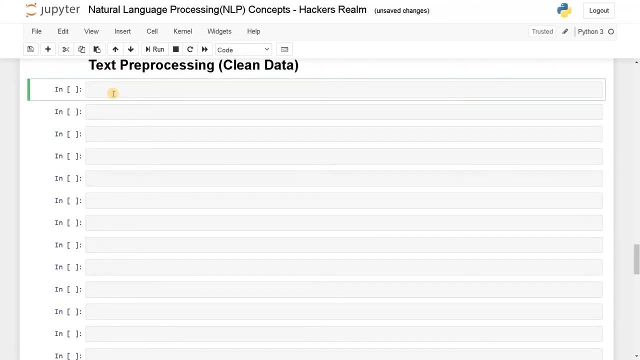 Hello everyone, this is Ashwin here. In this video we are going to see how to preprocess text data, So this is also considered as cleaning of text data. So I'll just have this here: Cleaning data. Okay, for this I'm going to load Twitter sentiment data. So DF equals. 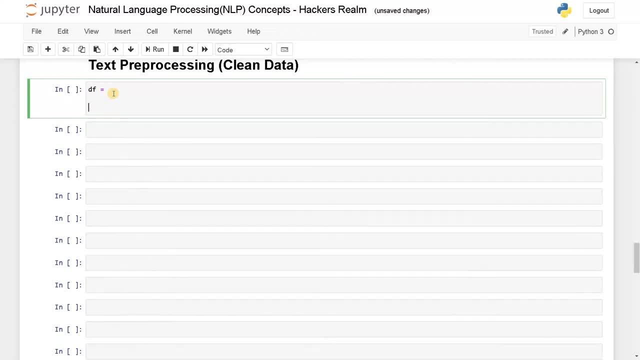 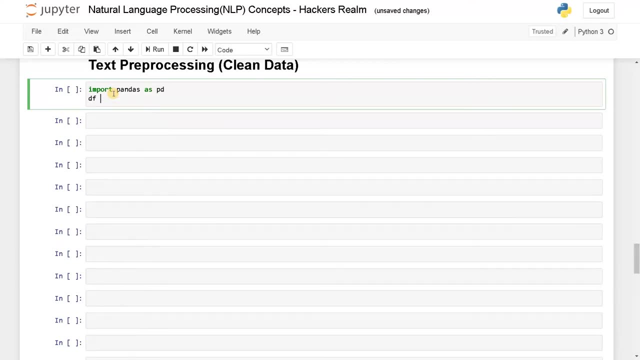 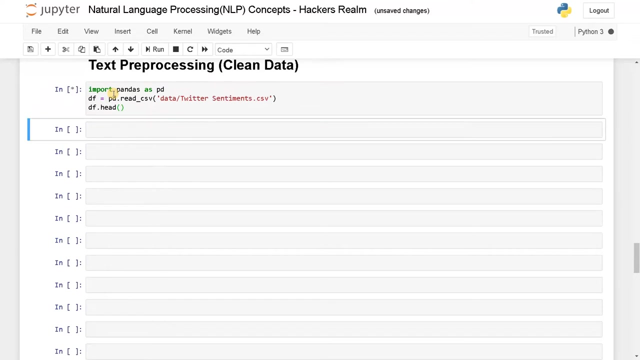 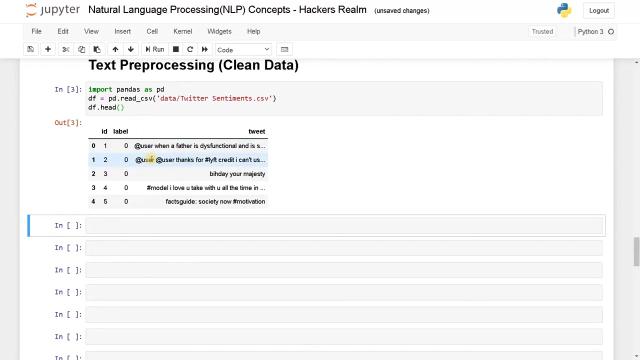 thing we have to import pandas first. Import pandas as Pd Now. DF equals Pd, dot read csv and data slash Twitter sentiments. DF equals pd, dot read csv and data slash Twitter sentiments. data slash Twitter sentiments: head run this now. this is the twitter sentiment data. we already done a project for twitter. 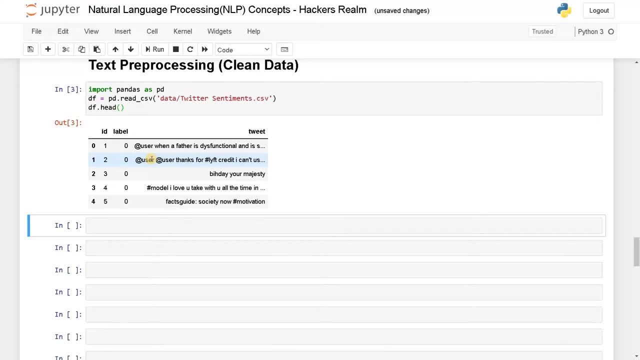 sentiments and we also done the pre-processing in that project as well. so for the tweets, i have done some specific pre-processing. if you want to watch that, click on the right top corner of this video to watch that complete project from end to end. now i'm gonna use this tweet for the entire. 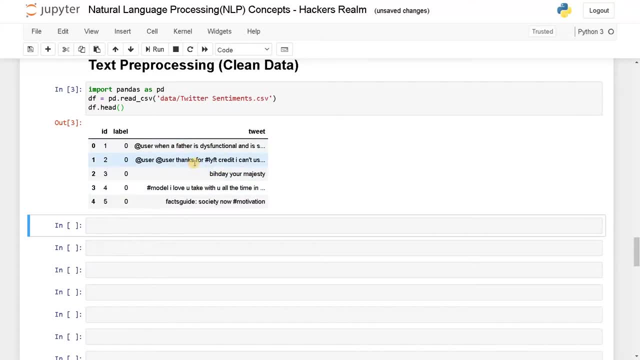 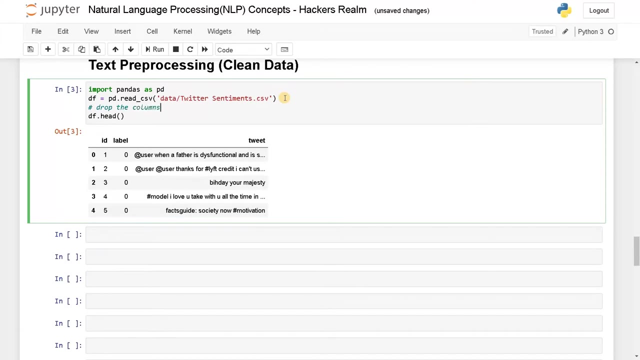 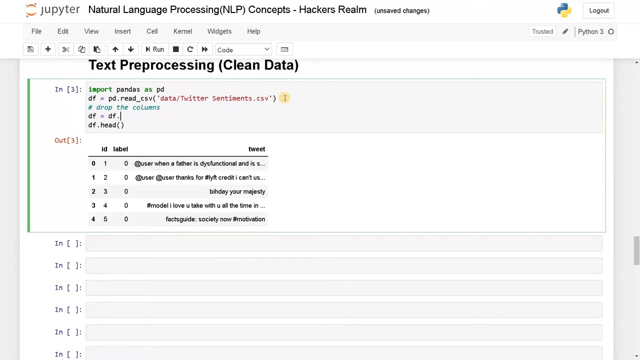 example for the text pre-processing, because it contains all the special characters and pretty much everything, and i'm gonna drop these two columns because we don't need that. so here itself i'll just drop the columns. so to drop that df equals you df dot. drop of columns equals. 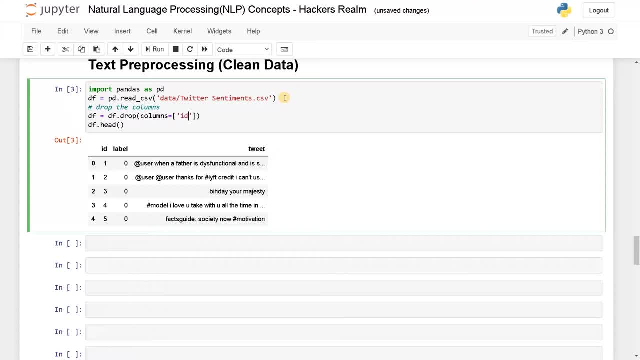 so i'll drop the id and label. access equals one run this. now we have only the tweet, so we can move to the next step. so the first step of every pre-processing for text data is to convert the whole text into lowercase. it seems like it's already in lowercase, but to be sure, we will just. 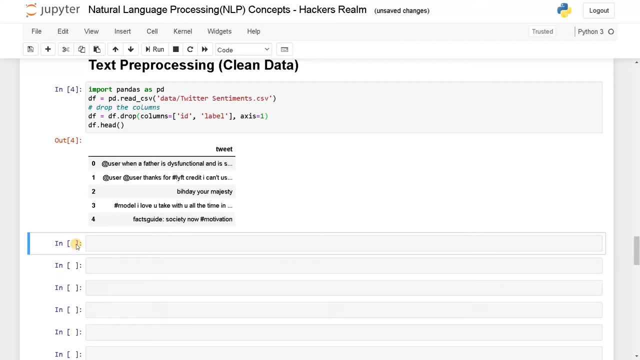 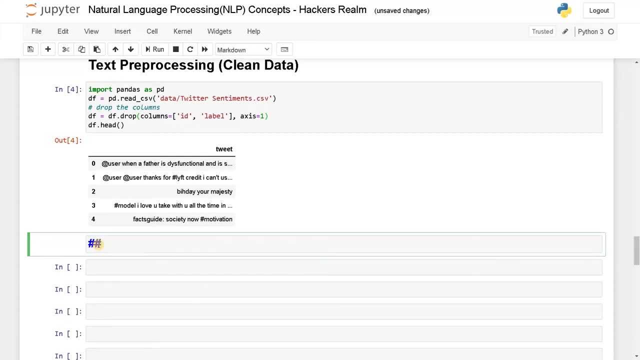 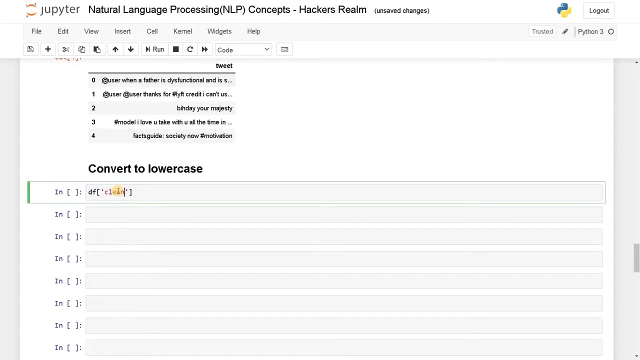 convert it right away. so this is the first pre-processing technique: convert to lowercase. so for this i will create a new column for storing the clean text. so clean text equals df of sorry tweet dot string. i'm just converting that particular column into a string in order to use that lowercase function, because the string already have some inbuilt functions for lowercase, now lower. so this is the function. it will just convert all the 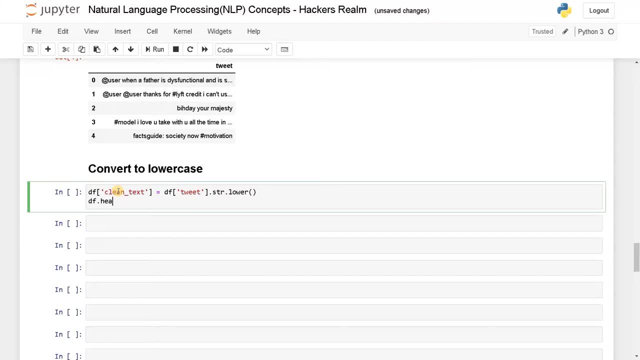 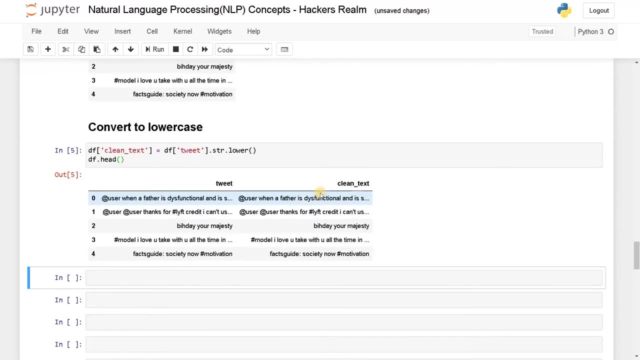 characters to lowercase Now dfhead. run this now. this is the clean text and for this example I don't have a text difference here. I think I may need to shuffle. maybe I will just use dfsample of fraction equals 1,. well, even after shuffling, I can't able to see any concrete evidence of like. 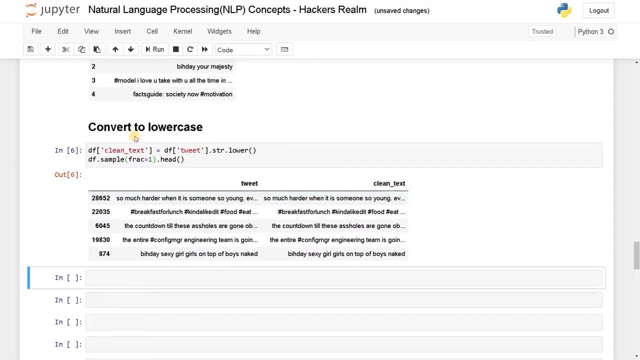 any uppercase or lowercase in the tweet. So this is a common step, so it will be much easier for the entire preprocessing workflow, so be sure to use this. and the next one is to remove all the punctuations, because we don't need this punctuation. 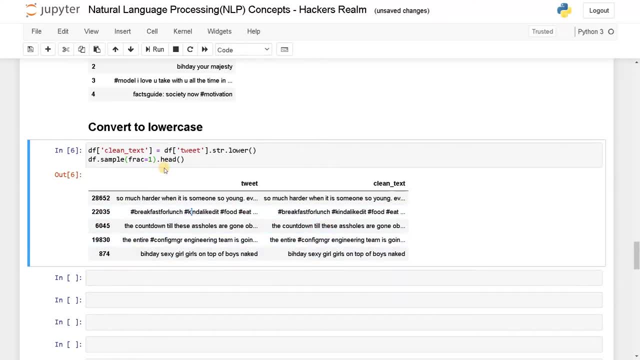 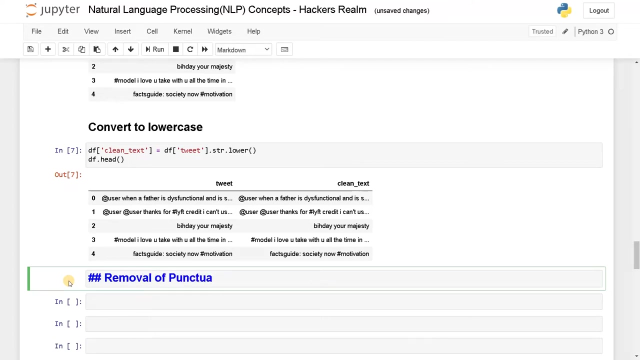 So there are, like many different punctuations we will be seeing in this data frame. I think I will just remove this for now. Now you can see all the punctuations. now let's remove that removal of punctuations. now for this, I am going to like create a function. 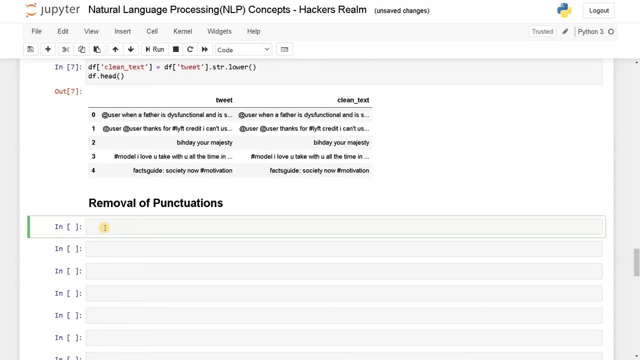 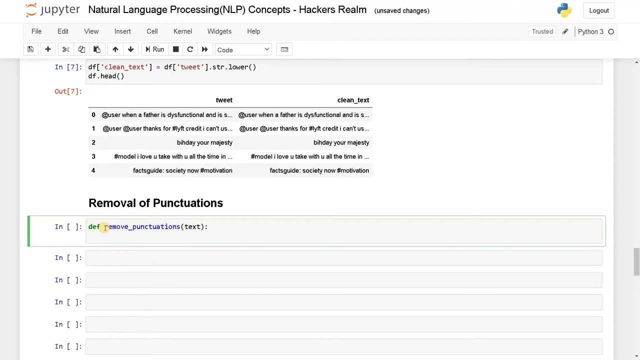 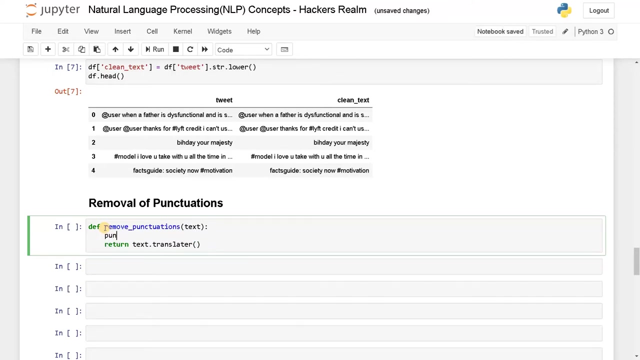 So it will be easier for us to do or even call the functions separately, if you want. so def, remove punctuations. just pass the text here and just written text, dot translate. Before that I will just stop. Okay, create a variable for getting all the punctuations. so here I'll just say: 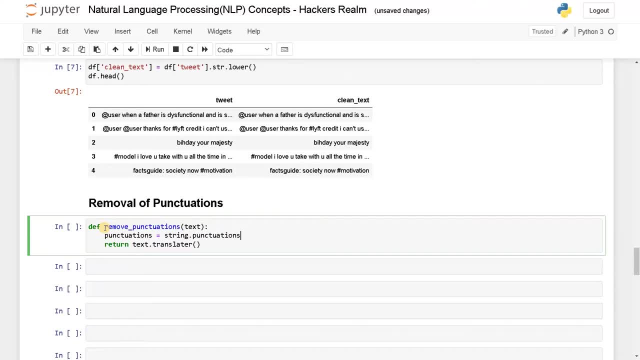 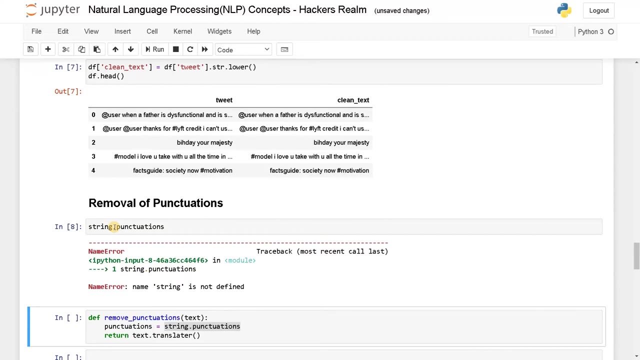 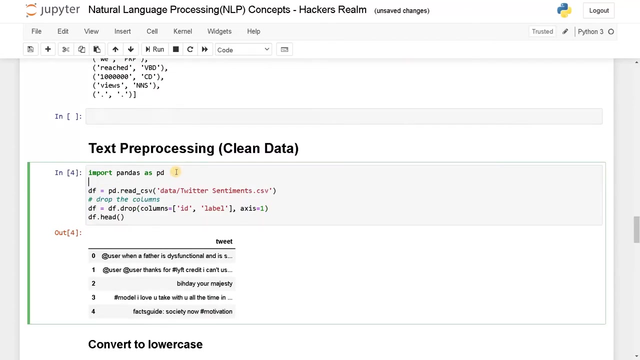 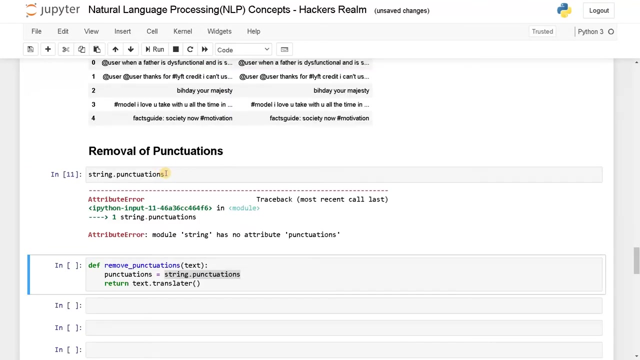 string dot. punctuation. I think s won't be there. okay, it's also having. yes, we can also display what are the punctuations available, so I'll just do it in a separate cell. okay, string is not defined. maybe I'll just define it here itself: import string: okay, okay, now you can able to see all the punctuations, so. 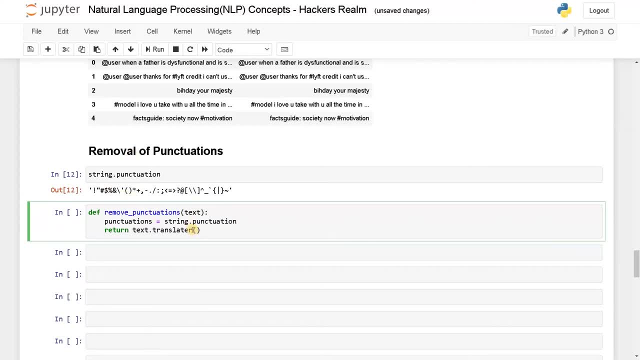 these are the punctuations we are going to remove from the text. now here: text: dot translate steer dot, make trans of empty character in an empty character. and what are the punctuations we have to remove? that is the punctuations now. this is the function. let's run this now. let's call the functions using DF dot, like apply. so 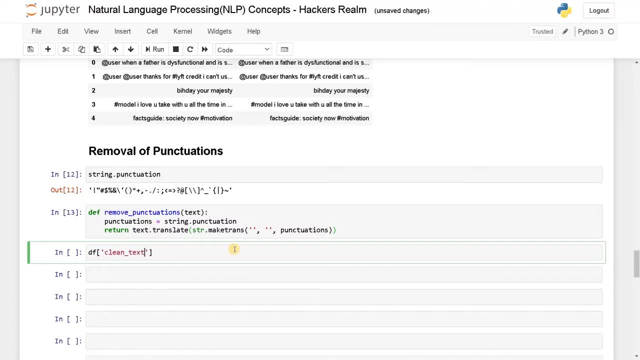 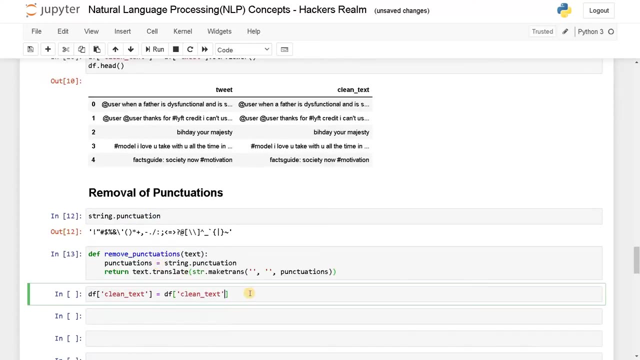 I'll say DF of clean text equals d � for yeah for this we will just take the clean text itself for further processing so clean text dot apply lambda so this is a common function we'll be using for pretty much everything lambda. tester is like a parameter and remove punctuation so off your 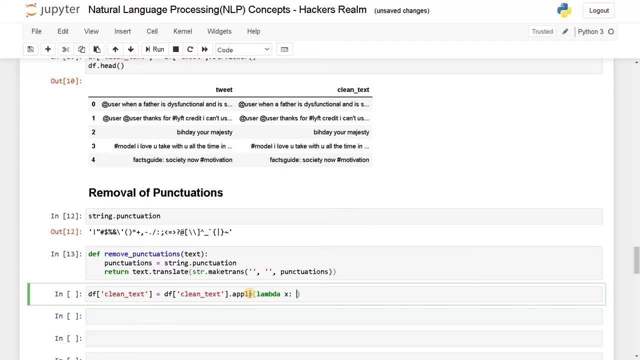 So this is a common function we will be using for pretty much everything. lambda X is like a parameter and remove punctuation of std parameter. so it removes an infinite number of punctuations. load untouchedile of a positive показ that or power x. so for each row it will just pass the sample as the x and we are just calling the remove. 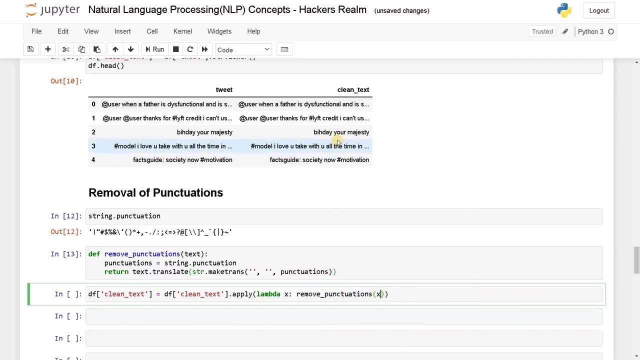 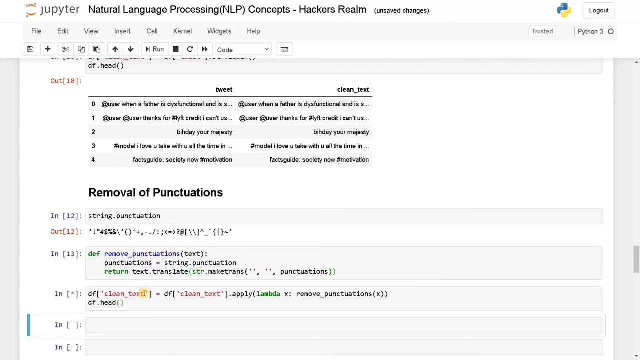 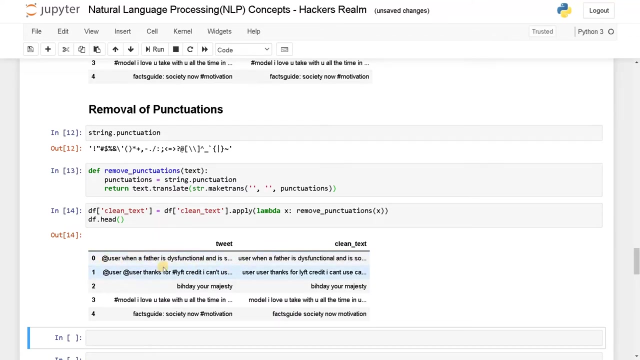 punctuations here of passing x, as the parameter x is nothing but the clean text. so it will just pass this and we'll be removing the punctuations here now. let's run this and display it as well. so df dot head. okay, now we can able to clearly see a difference here. so all the symbols has been. 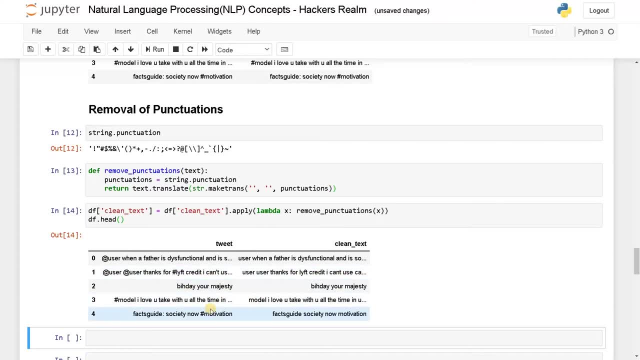 removed completely and the text is pretty much much better compared to what we have before. so this is the original text actually, and this is the pre-processed test and this is the pre-processed text. so i think this is some much more easier to process without all the punctuations, what we are having in the original. 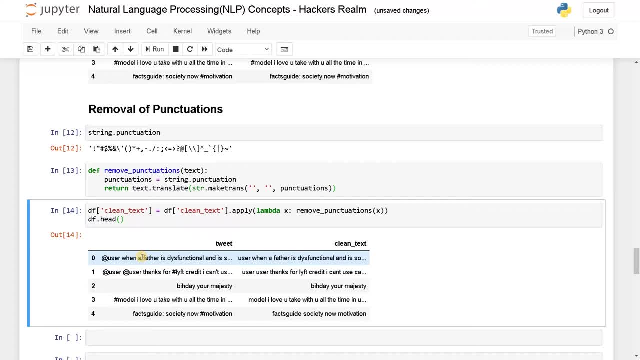 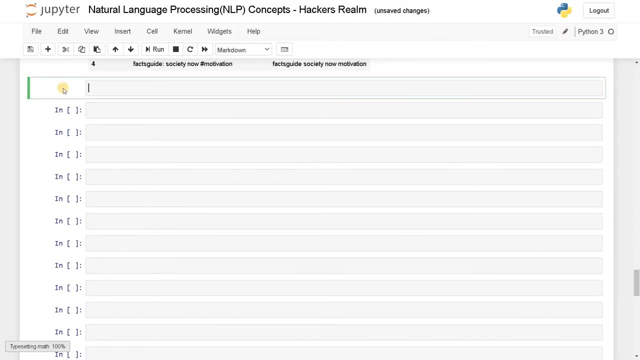 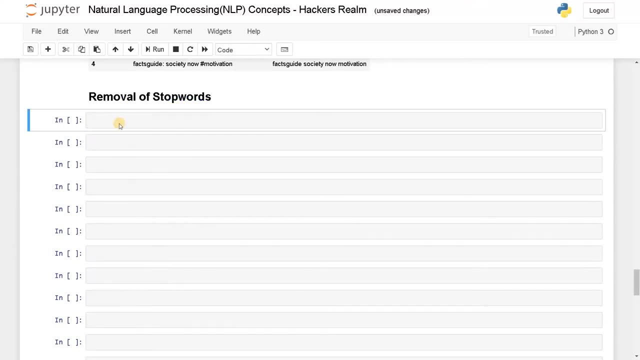 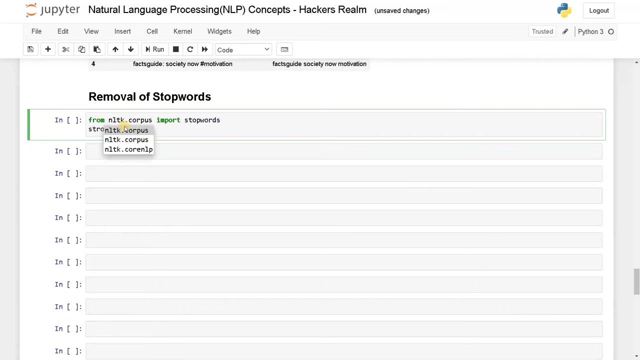 text. so this is one of the important functions, and after that let's go for removal of stop words. so removal of stop words: run this and the stop words is available in nltk library. so from nltk library, so from nltk dot corpus corpus, import stop words and stop words. 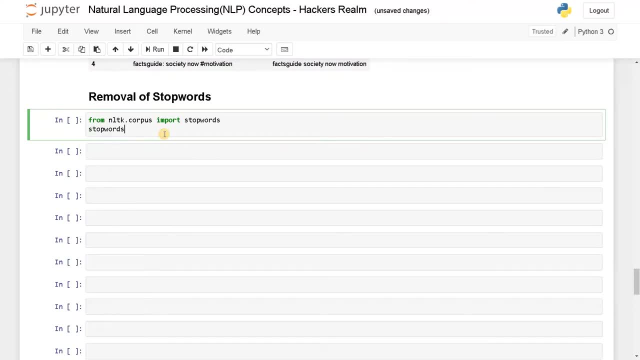 okay, stop words, dot words. you have to specify the language also, so i'm gonna specify english. run this now you can. you have to specify the language also, so i'm gonna specify english. run this now. you can see all the stop words that are. see all the stop words that are available. 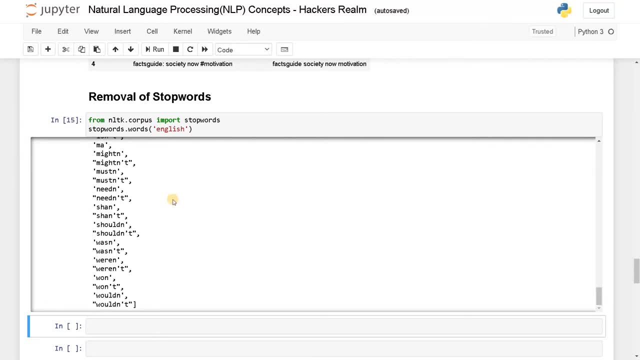 available. uh, these are like uh pronouns, so we are. uh, these are like uh pronouns, so we are just uh. trying to remove all the pronouns that are like just uh, trying to remove all the pronouns that are like frequently occurring, so it will be easier. 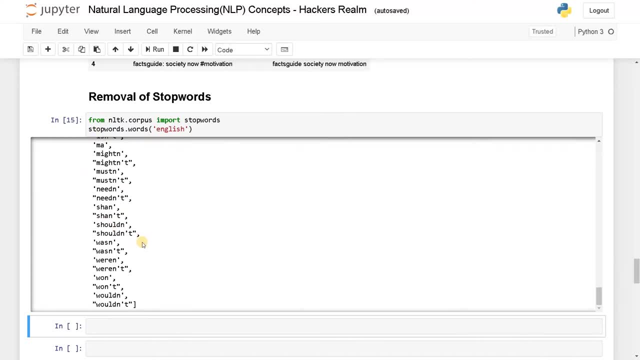 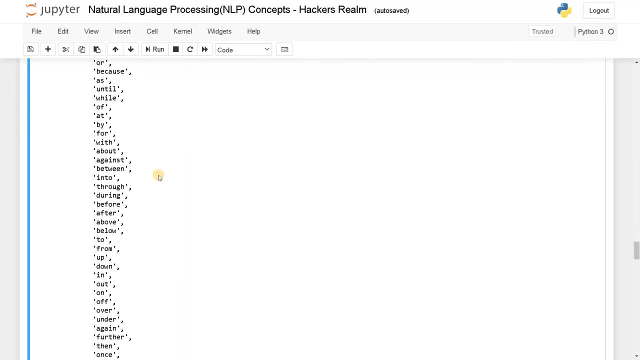 frequently occurring. so it will be easier for us to do the processing. so we'll be removing all the for us to do the processing, so we'll be removing all the stop words available in the text. i think if you expand, it means it will be like a bigger stop words, if you want to simply see that. 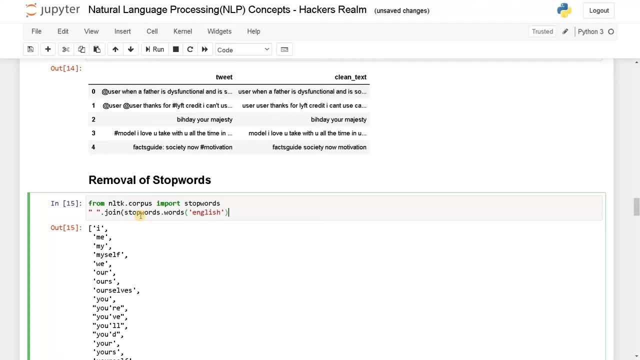 i think if you expand it means it will be like a bigger stop words if you want to simply see that you can use. i think if you expand, it means it will be like a bigger stop words if you want to simply see that you can use dot, join off. 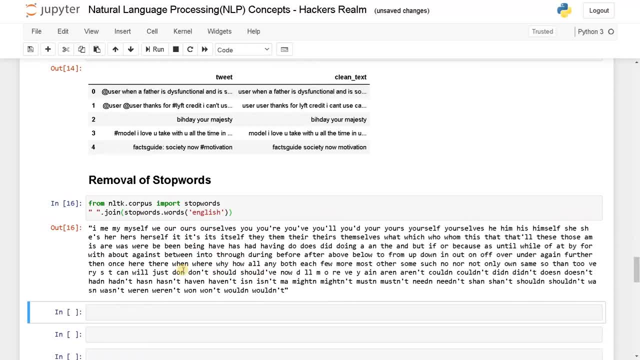 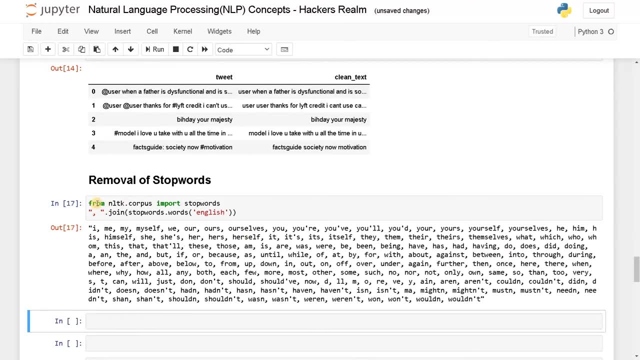 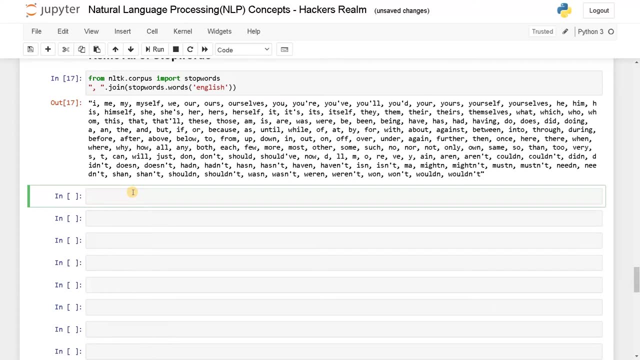 stop words. okay, now you can see all the stop words with the space, or you can have a comma, so it will be clear for you. now we'll be proceeding to remove the stop words. now we will create a stop words variable, so usually we will just create a. 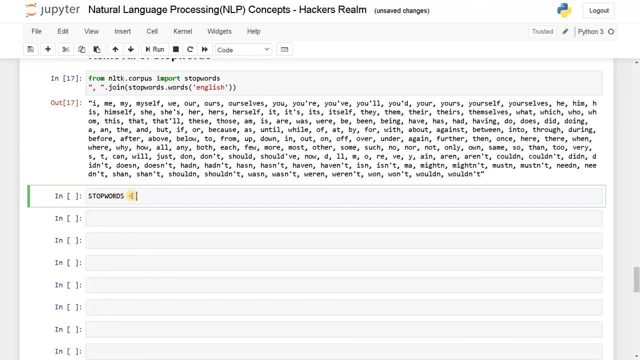 variable. so usually we will just create a kigtel words like stop words equals kigtel words like stop words equals set of set will just remove the duplicates. set of set will just remove the duplicates if they have any. if they have any, and it will be easier for two. 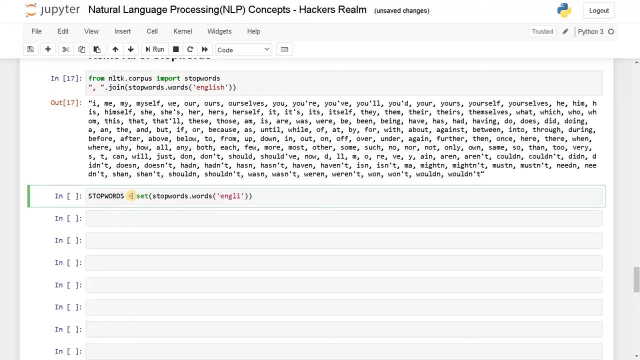 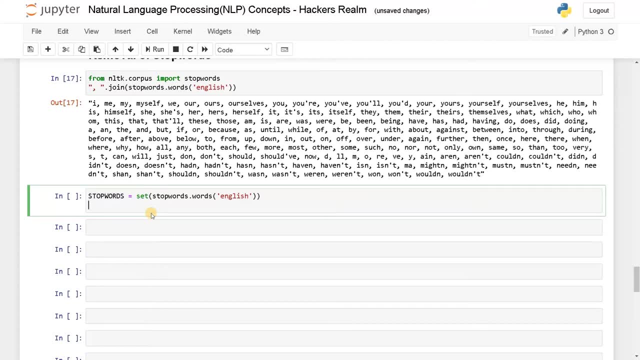 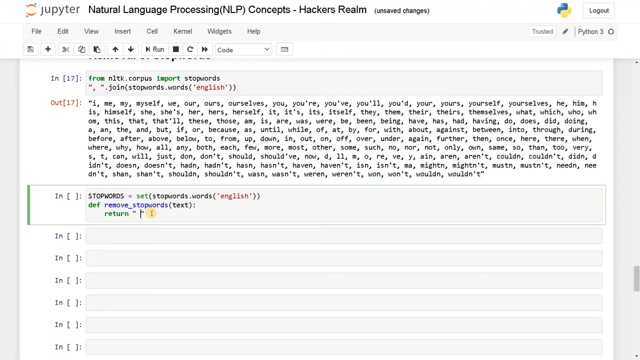 get the unique stop words english. now this will have all the stop words in a set and again we will just create a function. so depth: remove stop words, gain text here written dot, join off in a list word for word in string of. I think we'll be just passing that text So x, dot, split And if word not in stop words. 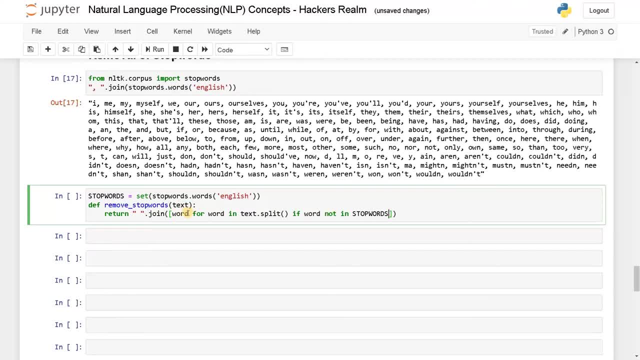 so if they're not words not in stop, what's means? it will append it to the word and we'll be having all the sentence. So what it does is it will just remove all the stop words if it is present in the sentence. 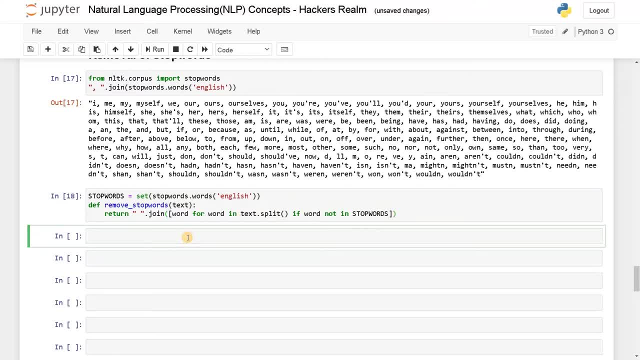 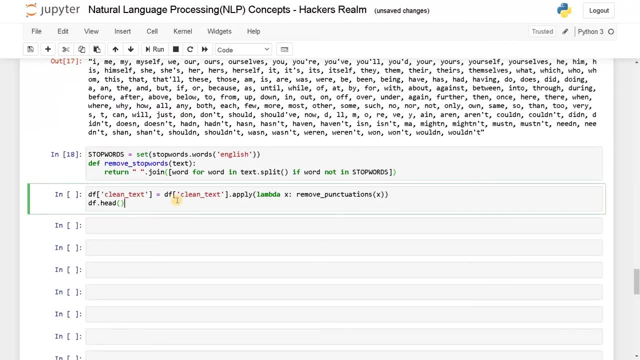 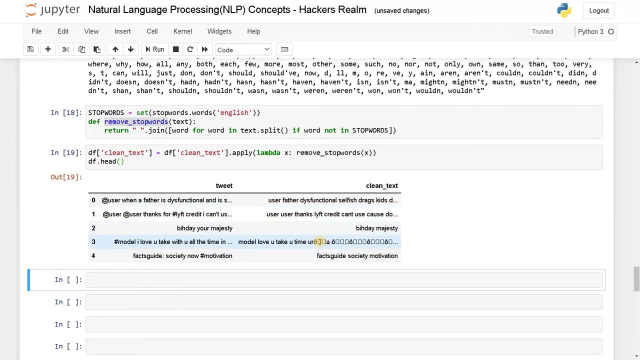 So this is the whole function And again we will just use the same syntax. Instead of remove punctuations here, it will be remove stop words. Okay, let's run this. Okay, we have removed pretty much all the stop words, And these are some emojis, something like that. I guess Can't able to get it. 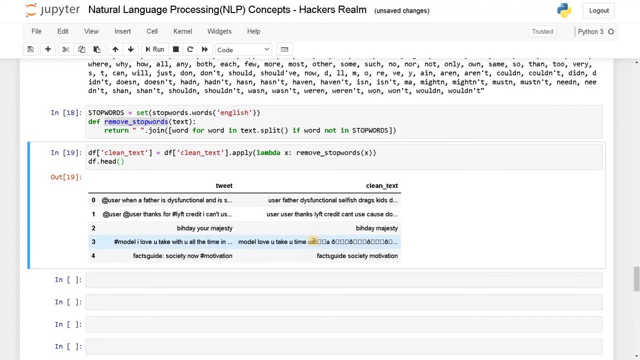 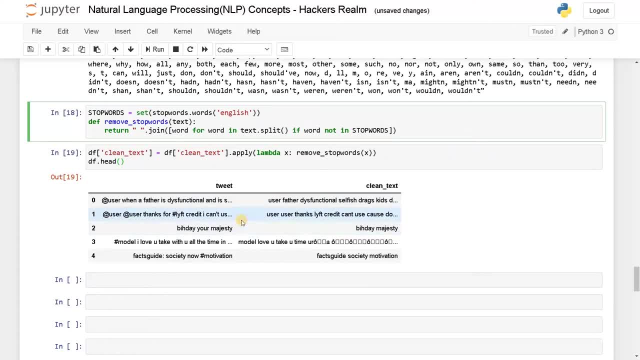 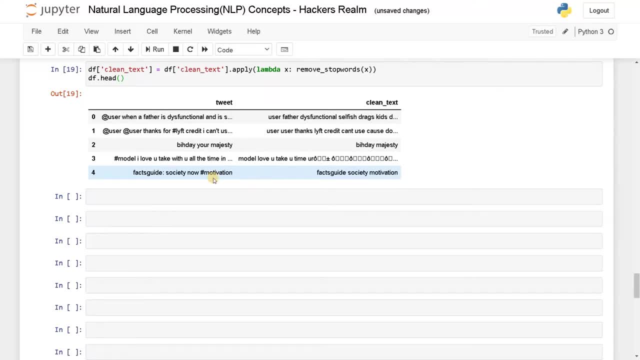 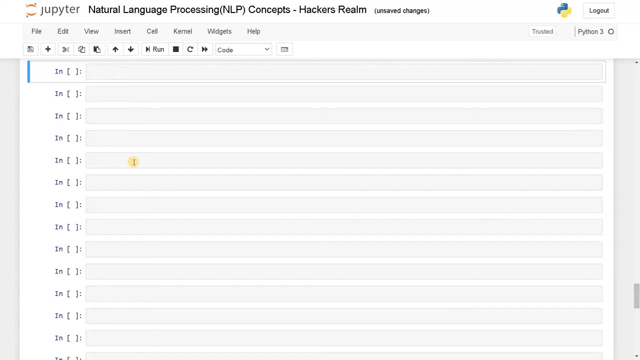 is the advantage of using our stop words? it will just remove all the frequently occurring pronoun, So that won't contain like that much meaning if you are dealing with machine learning project. Now, after removing stop words, I'll just go for removal of frequent words. 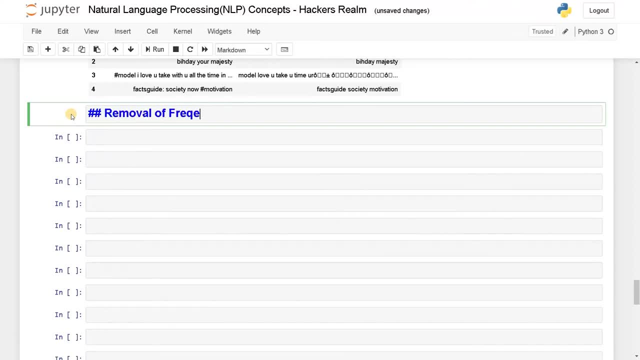 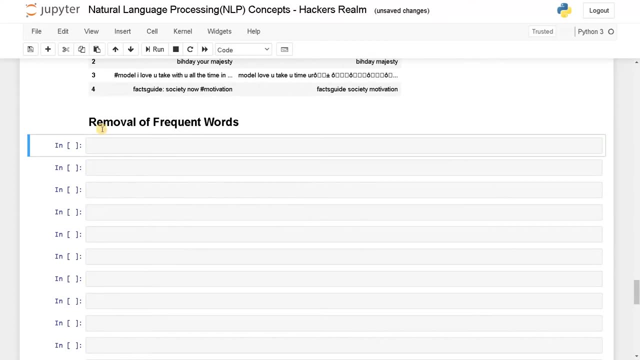 So removal of frequent words. okay, now I'm just gonna remove like the top 10 words from the whole corpus. it's not related to like stop words, but some other words that are. normally it will be keep on occurring, so it's better to remove most frequent. 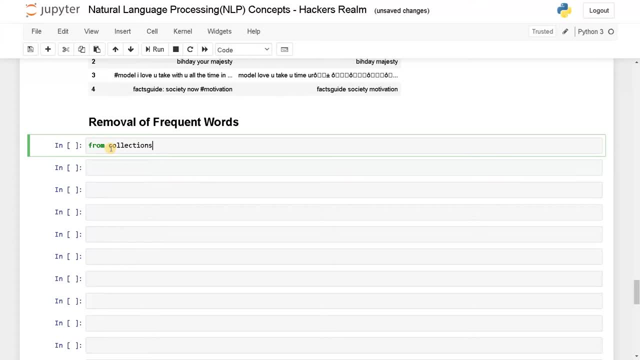 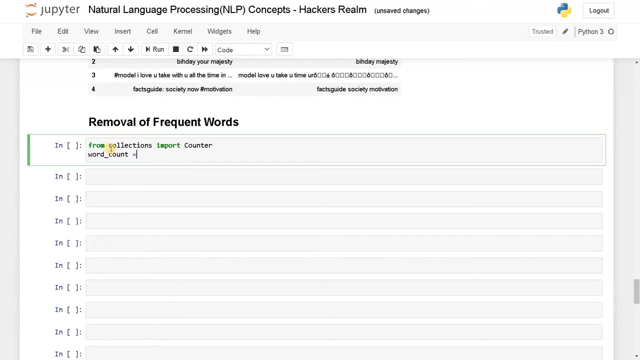 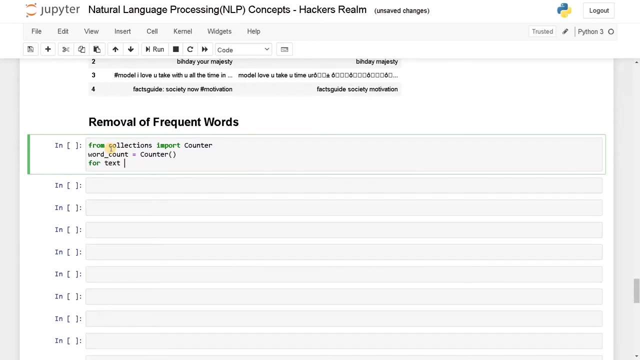 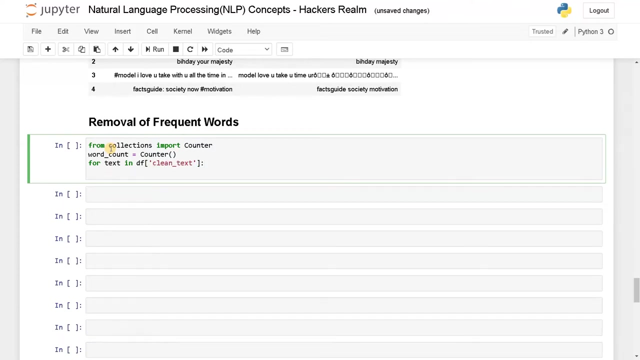 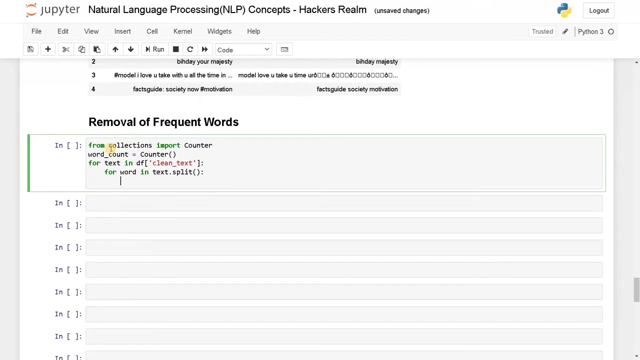 words. so for that from collections import counter I will create word count equals counter, just initializing like a dictionary. so for text in df of clean text, now for word in text dot split, here we'll be using word count of text plus equals 1 if the text is not present. 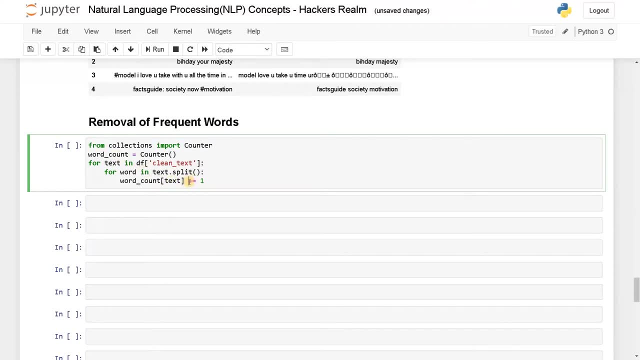 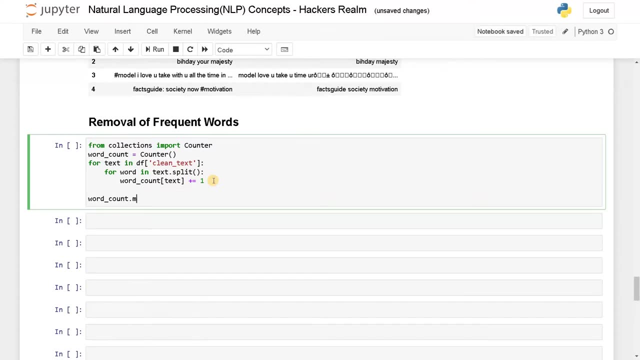 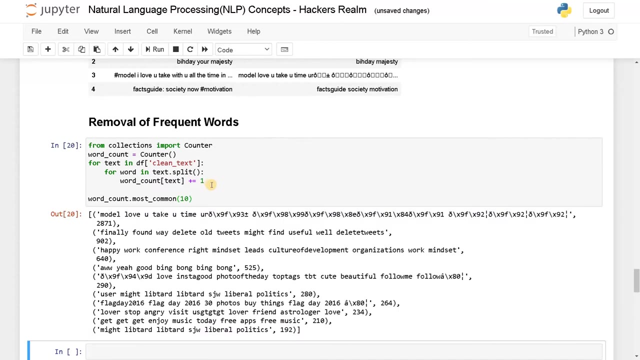 in the dictionary means by default, it will have 0 and we're just incrementing the count by 1 and after doing this, I'll just display the most common. most common, like 10 words that are frequently occurring. okay, I think that's it for this video. I hope you liked it and if you have any other questions, 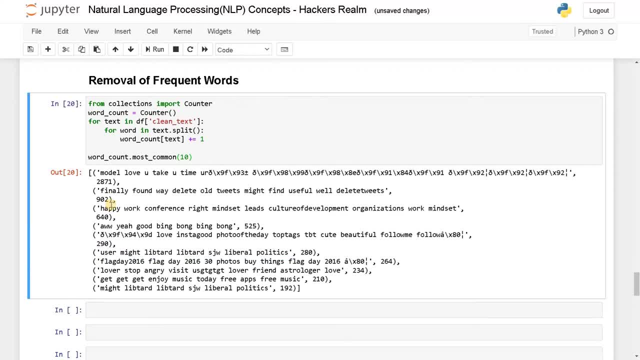 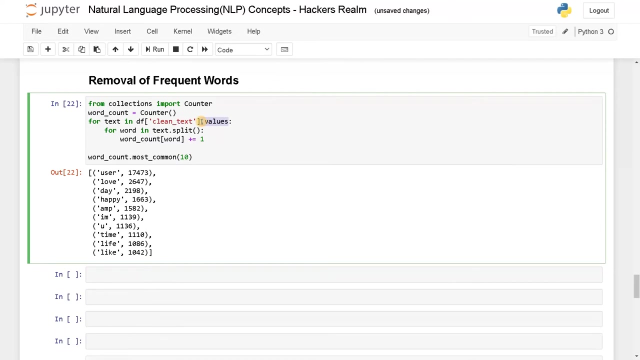 please do. let me know in the comment section below and I'll see you in the next video. bye, bye. I think it's taking the whole thing as a string. maybe I'll just say df in text, dot values. okay, here it is word. now let's run this again. even we can remove this, okay. so here you can. 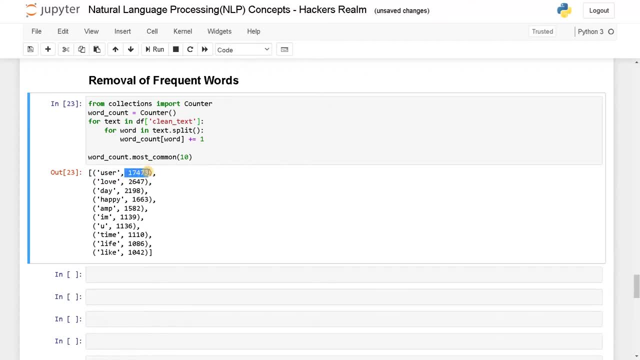 see this, you will. user is like a string and it's taking the whole thing as a string. now let's run this again. even we can remove this, okay. so here you can see this user is like showing like 17,000 times. it is not not much important for us and all the remaining words. 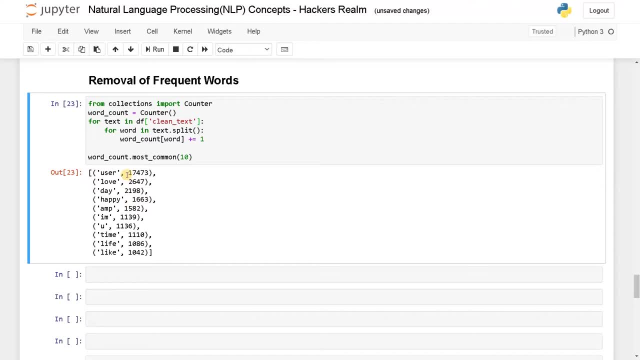 also like frequently occurring. but if I want to remove the one word means this is the word for this data set, that is user, and you can also see and remove all the words as well, and I'm just considering to remove only the words that are like in the top three for this. 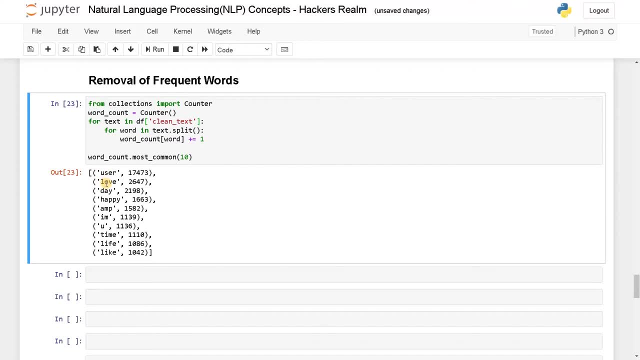 dataset. Uhh, So you, if the data you have is like somewhat meaningless, means so you can remove the whole top 10 also, that is your wish. So now let's remove the top three words for the data set. So I'll just create a variable for frequent words. equals, set of word for word, comma, word. 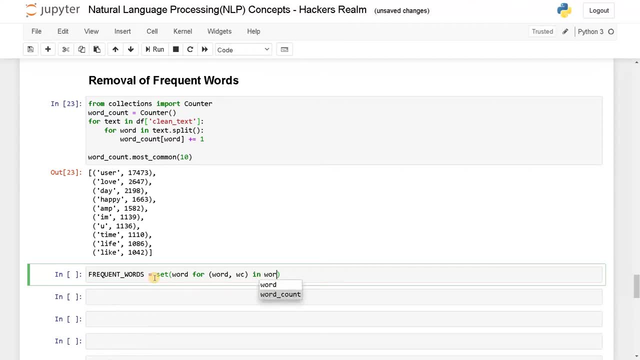 count in word count. dot. most common of three. So you can change the number if you want. You can change the number. You can change it to 10 as well. After getting the frequent words. I'll just remove frequent words, So I'll just create a function. free quotes of text: again written dot. join whatever we. 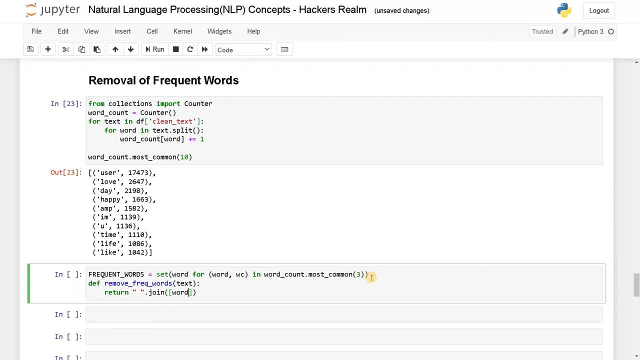 have done for the stop words, we are going to do it again: word forward in text, dot split. If you are interested, you can use this function for that. We are going to just do a few simple things here, So written in word and not in frequent words. 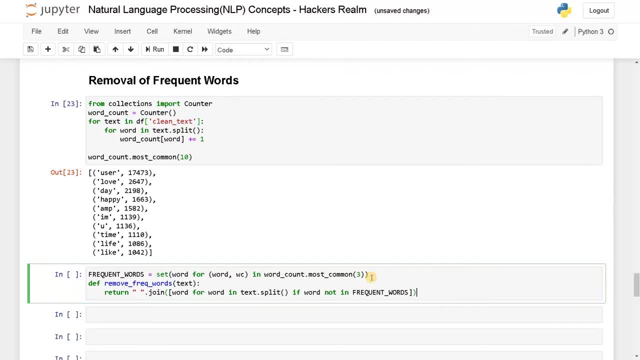 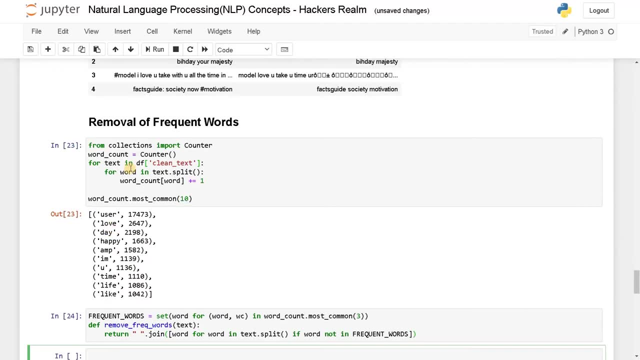 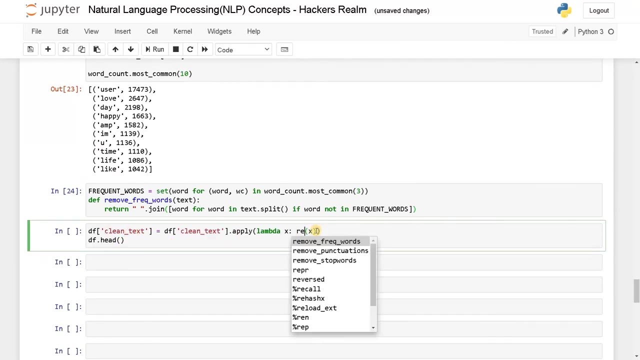 We will just write it as word in, not in frequent words. Okay, that's pretty much it. Let's run this once and here we will copy the same thing, Paste it, and here we will just remove the frequent words. run this. 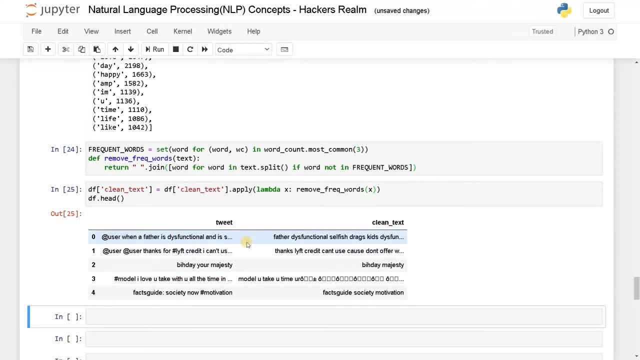 Okay, Now you can see we have removed the. Now you can see we have removed the frequent words: Hold on, Hold on all the frequently occurring words. this all the users has been like- removed completely. and love is also removed and day is also removed. so these are the three words i am just removing from this. 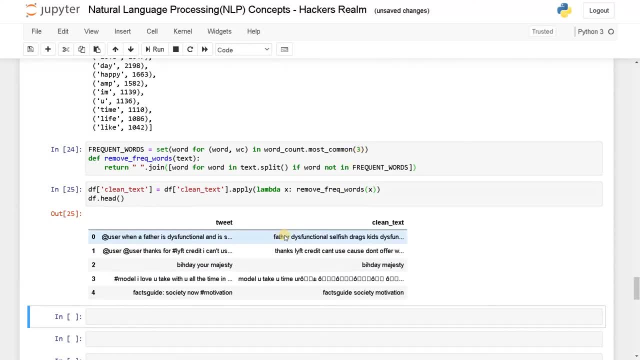 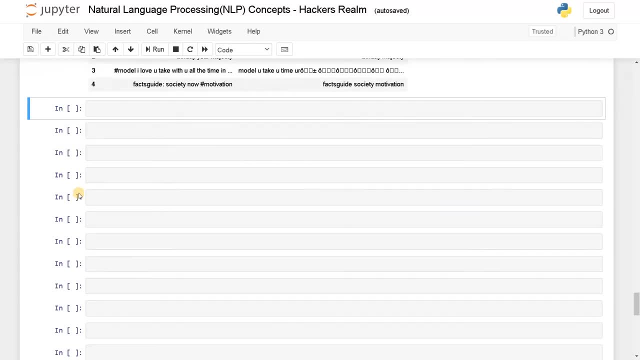 data set and, as i said, you can also change. this number depends on your data set. after that, we can also remove rare words. so that is like like not contributing that much to the data set, like we have only few words in the entire corpus means we can remove that, so for that we just have a. 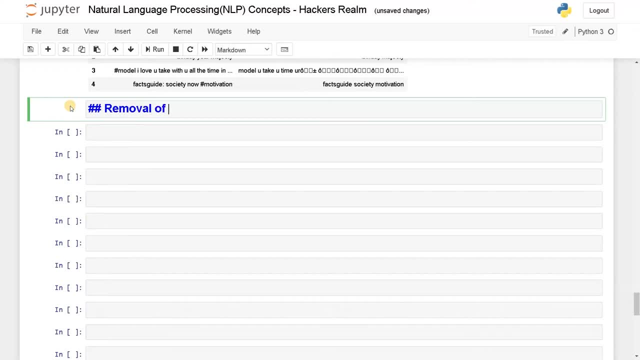 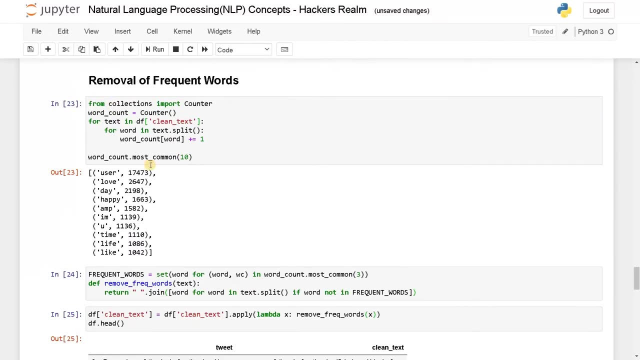 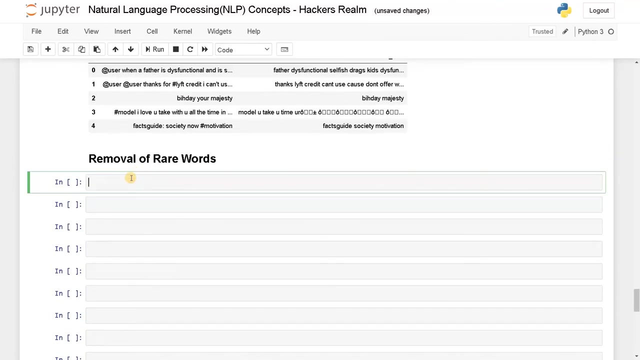 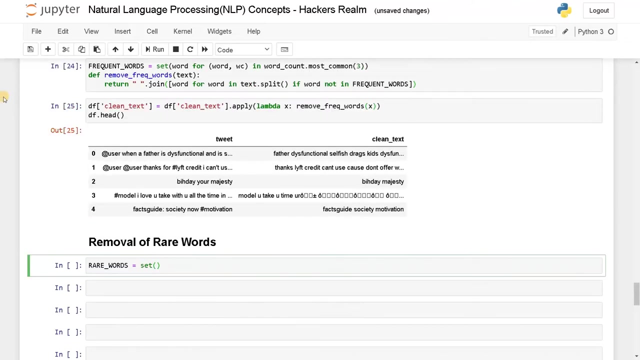 function similarly. removal of rare words. okay, you can use the same word count instead of using the most common. i'm gonna go for like least common. for that we have to filter out few things, so i'll just say a rare words. rare words equals set of. i'll just copy and paste this because that's pretty much similar. 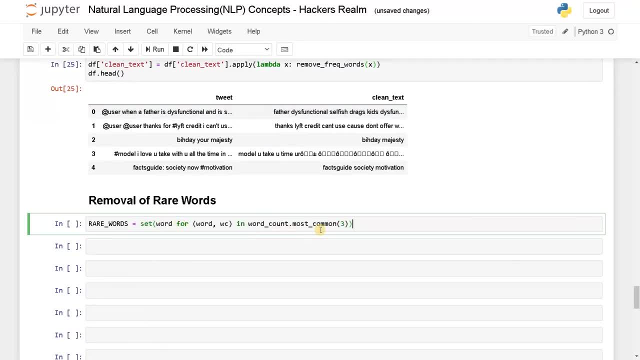 okay. so here, uh, why, when we are getting that uh most common, i just have this: uh 10. sorry, in the most common i'll just take everything and here i'll just say minus 10 and minus 1, so this will get the least common, like the least occurring words. 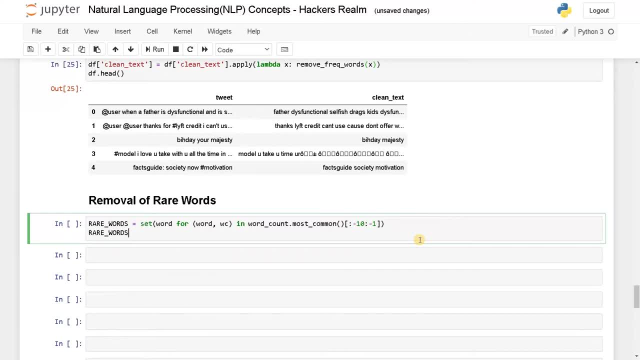 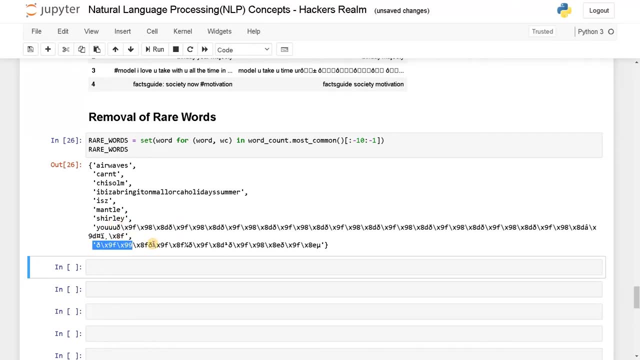 you can also see the words: if you want食 absorb, run this. so this is the least occurring word. i think these are all like some kind of a special characters. we can also remove this, so it may be a emoji or some kind of a emoticon like this, because in twitter 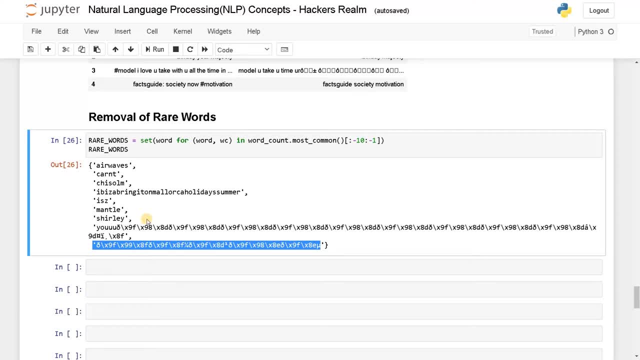 it also available and the data set may also contain those kind of special characters. we'll also see how to remove those as well. currently, i just considering these other words that are considered like rare. you can also see the count um for that if i display it as like this: 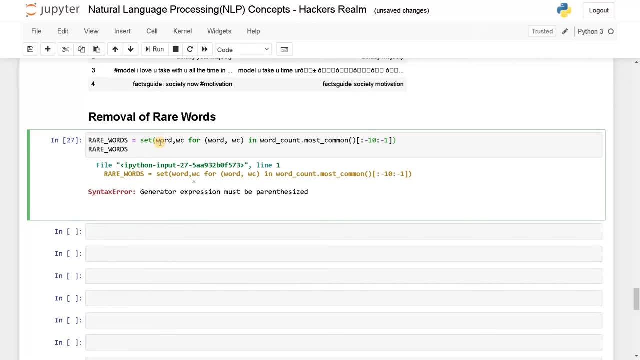 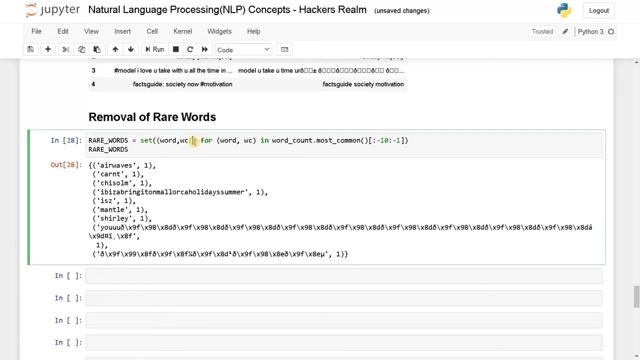 i don't know whether it work. no, it's not working. i think i have to make it as like a tuple itself. just to see the count. i'm just uh having this: okay, everything is just occurring like one time only, so we can uh clearly remove it. just to see the count. i'm just having this: okay, everything is just occurring like one time only, so we can uh clearly remove it. 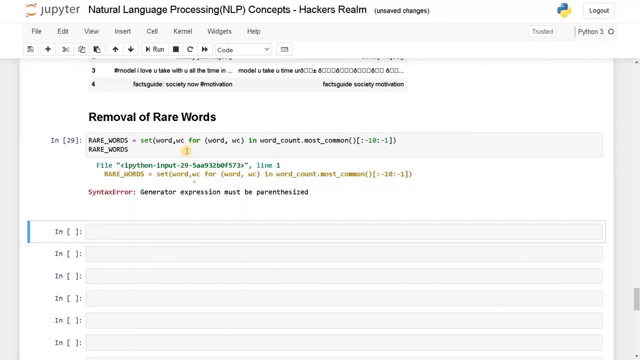 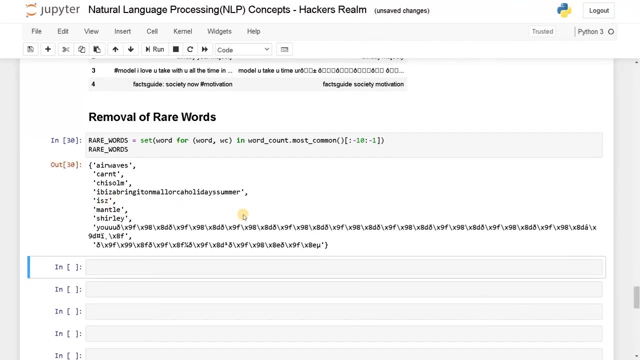 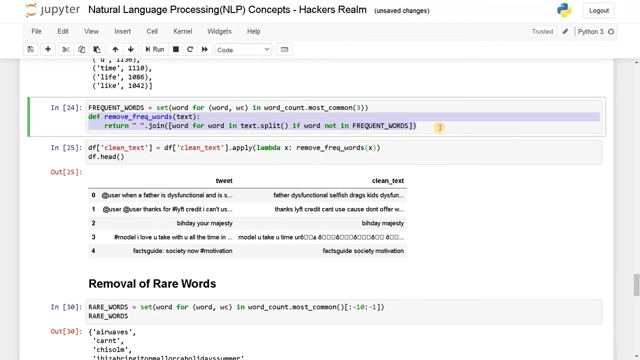 okay, everything is just occurring like one time only, so we can, uh, clearly, remove it. okay, run this. okay, i again done this. okay, so these are the words we are going to remove, and again we can use the same thing like: instead of this, frequent words, i'm just gonna go for rare words. 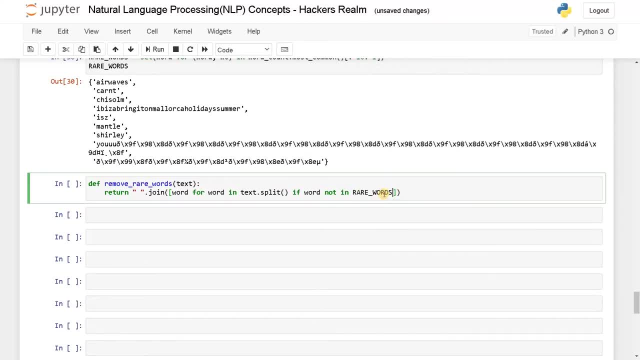 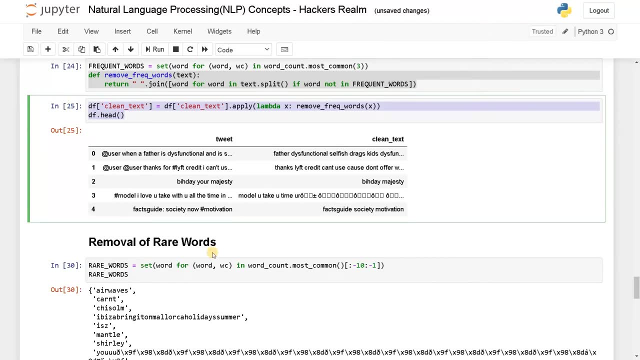 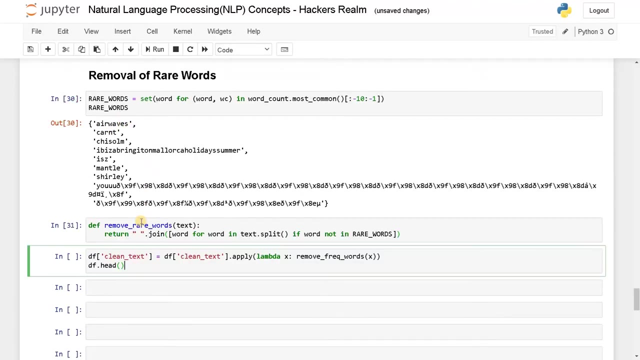 rare, rare. so this is the function let's, let's call this, but we can't able to visualize, uh, what are the words we are removing, because it's just occurring like one time. so like this, you can remove so many words from the corpus. you can remove like maybe 100 words as well if you have like a big corpus and all the counts. 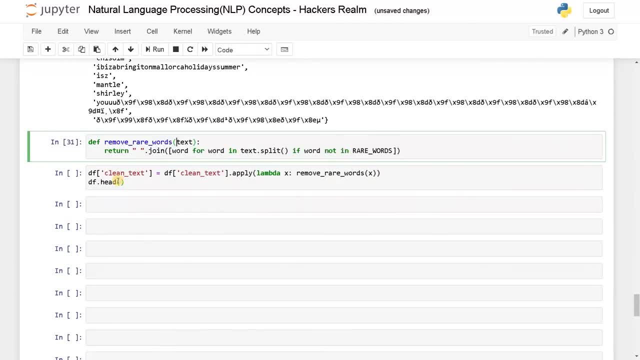 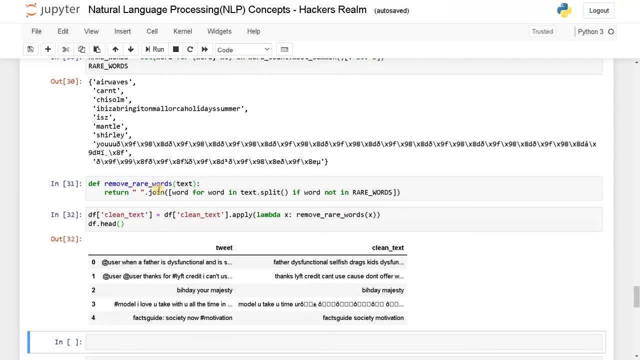 are having like less than one. so this is how you can able to remove rare words. run this. so this is how you can able to remove rare words. run this now. that is done. so now you can able to see some special characters to remove that. we will have a regular expression for that. 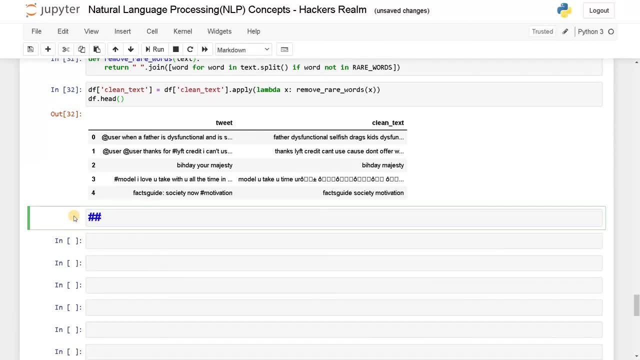 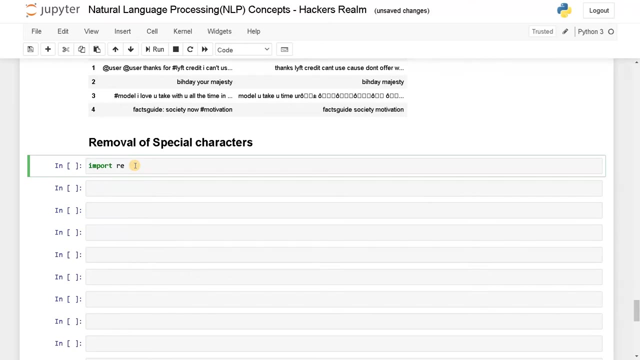 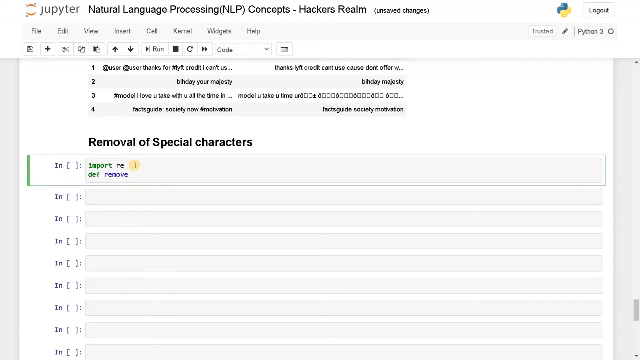 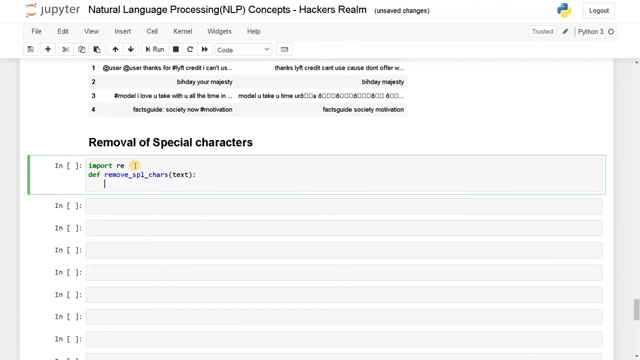 so this is like a shortcut. you can just directly jump into it if your data set is like that. so i'll say: removal of special characters. okay, now for this. i'm going to import rejects and i'll have a function: def: remove specialนะคะres. we'll just pass the text. so now, text equals. 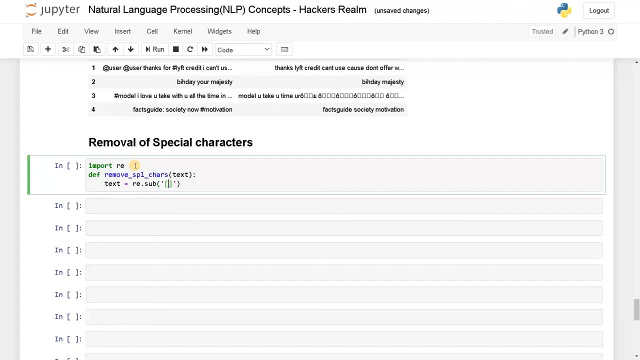 3 dot sub of. so here i'll just pass except a to z to set 0 to 9.. So what it does is it will just ignore the characters that are present in the range of lowercase a to z and uppercase a to z, and 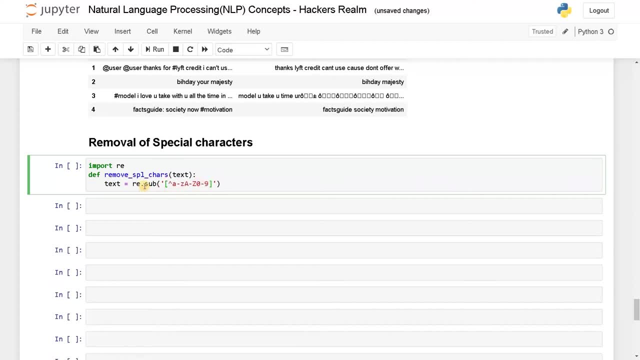 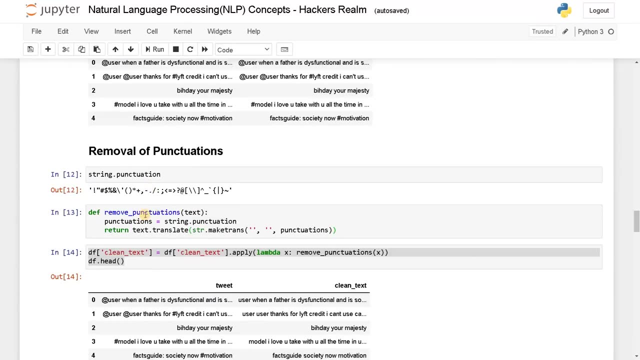 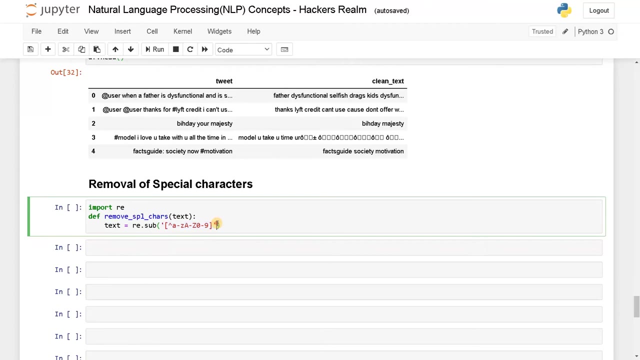 Finally, the digits, like 0 to 9.. So, apart from that, it will just remove whatever you are seeing, so you can just ignore all these things like this removal of punctuations and And Other special characters. you can just easily remove it like this. so here, just pass the text and 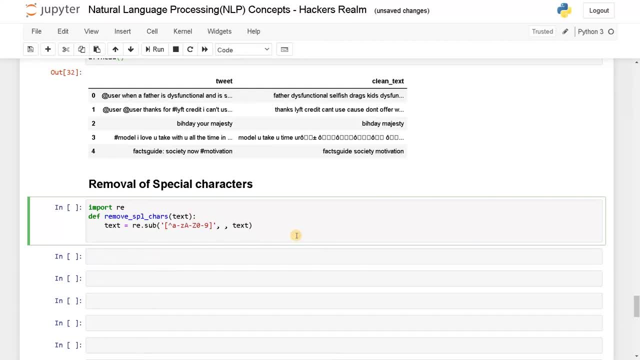 Okay, when you are doing this, you have to Substitute with something, so it will also remove the spaces. That's why I am just having the space here and After that, if you have like additional spaces means Read out, sub off, backslash, Okay, backslash s plus. 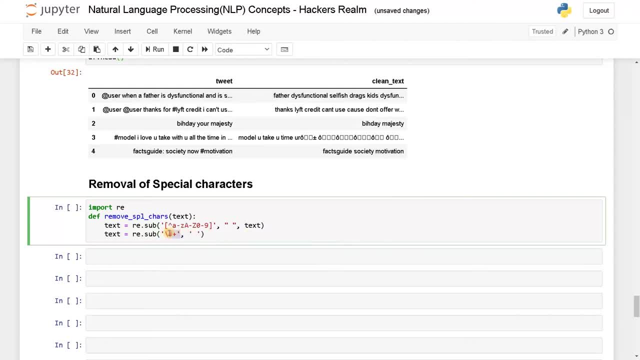 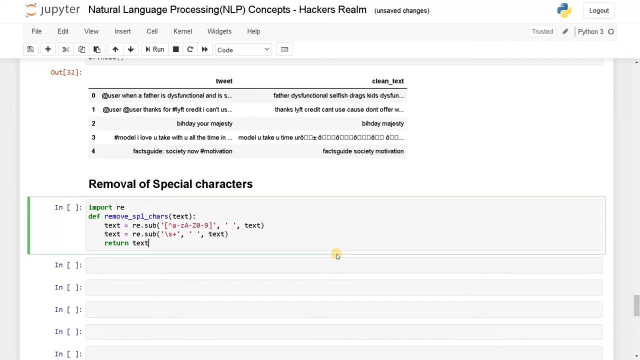 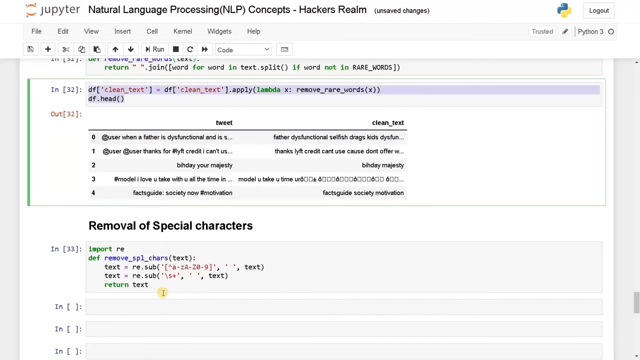 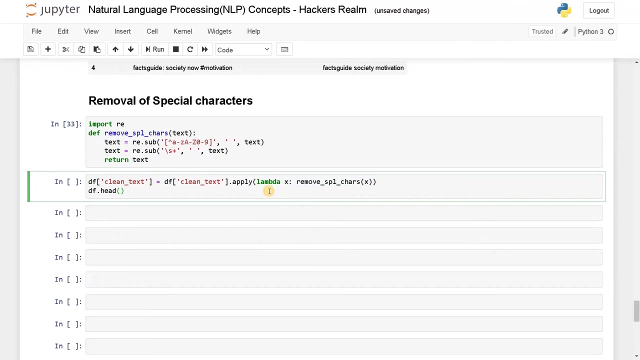 So this will just replace Additional spaces with like a single space. So this will be helpful for you if you are dealing with like additional spaces and Pass the text now written text. So this is the removal of special characters. Let's try this, Okay. Okay here. removal of special cars. let's run this. 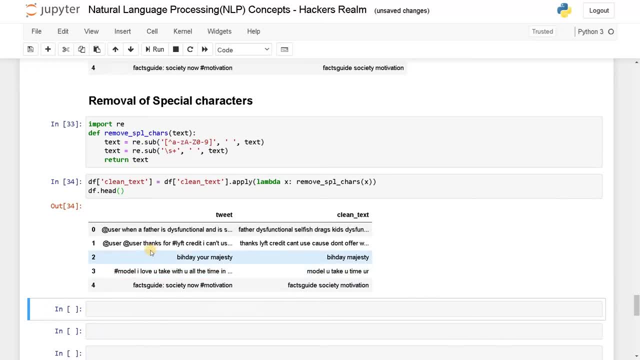 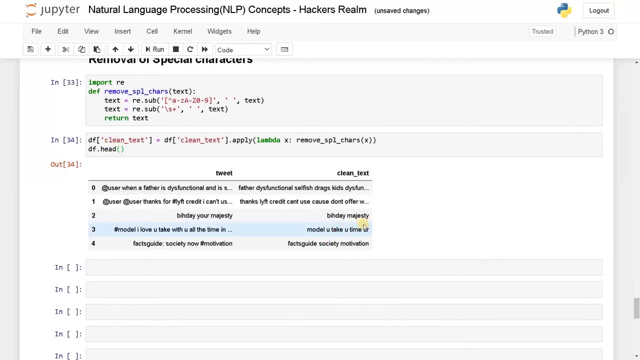 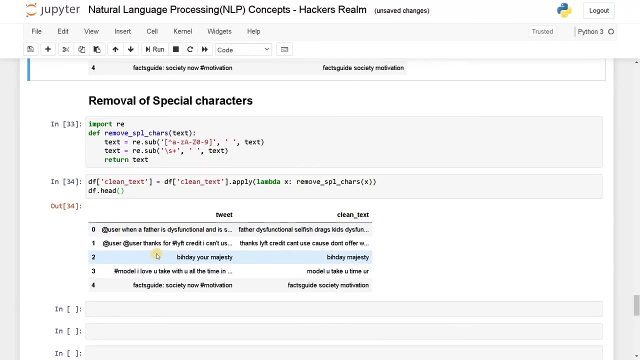 Okay, now you can clearly see We have removed all the special characters that have been there before like this. So we have removed everything and The text looks much cleaner compared to what we have in the original Tweet. So using this, you can easily pre-process or. 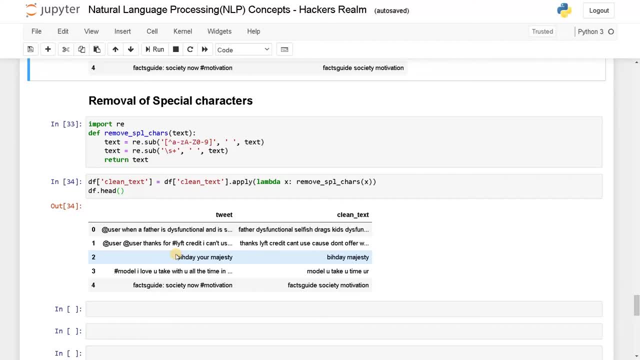 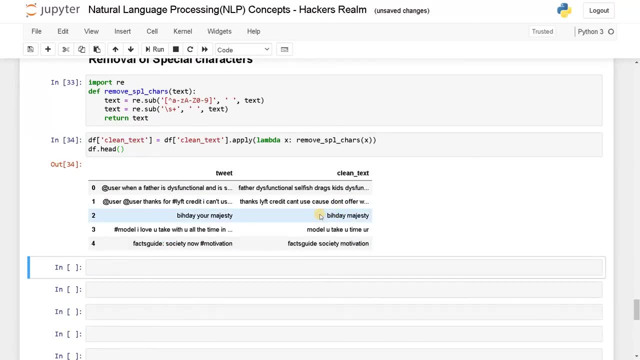 Do the normal Pre-processing techniques like word tokenization, Stemming, lemmatization. now you can proceed like that. Okay, after this you can easily go for stemming or lemmatization, now that we have a clean text. So again, I will just go for a stemming first. 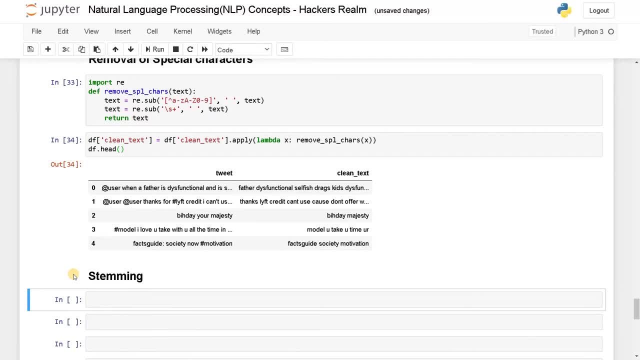 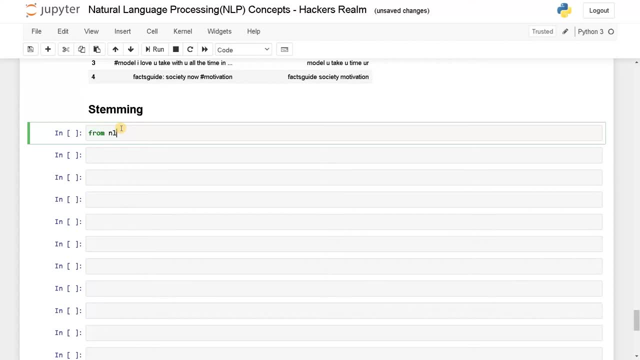 Here you can see that I have already created aule system Stemming. we already seen this in the previous videos, like how stemming works. You can also check that in the playlist. so for this I'll just import from an ldk dot stem dot port Porter import. 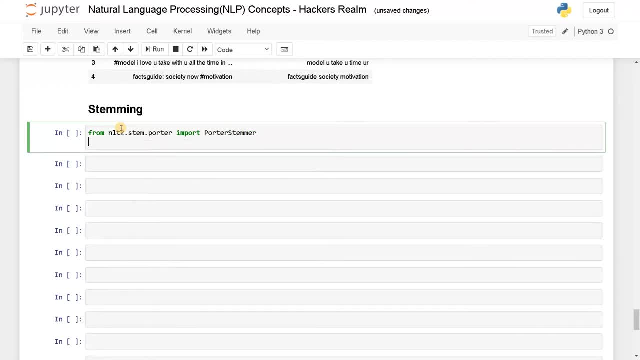 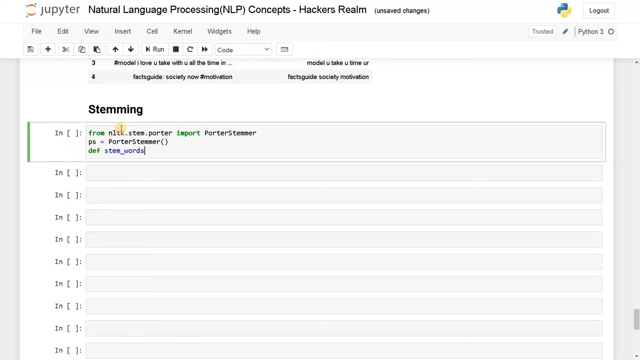 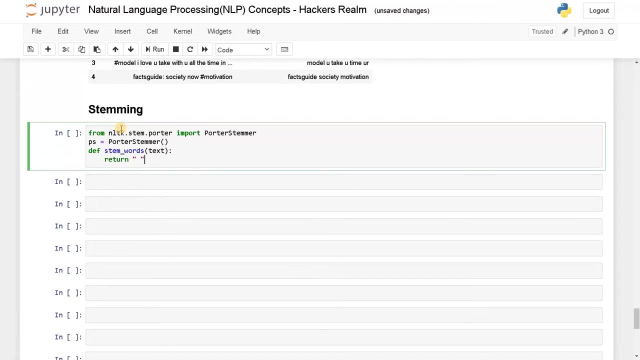 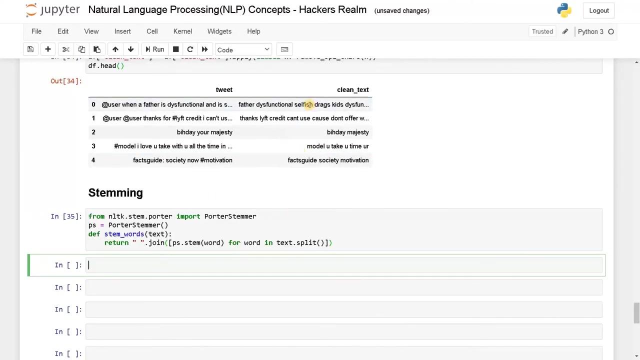 porter stemmer and Initialize it. Just call it as like PS itself, a stemmer, and here we will just stem words. text now written dot. join of again list: ps dot. stem of word for word in text, dot split. so this will do the trick, run this. so for this i'm. 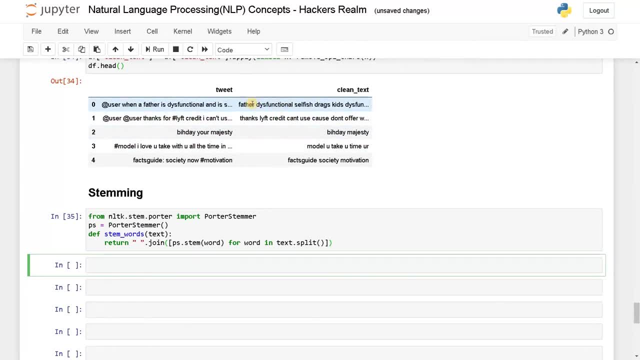 going to create a new column because we we just want this for lemmatization, because you can either use stemming or lemmatization for this data set pre-processing. it depends on your analysis or your scenario, so i'll just create a new column. so df of stemmed. 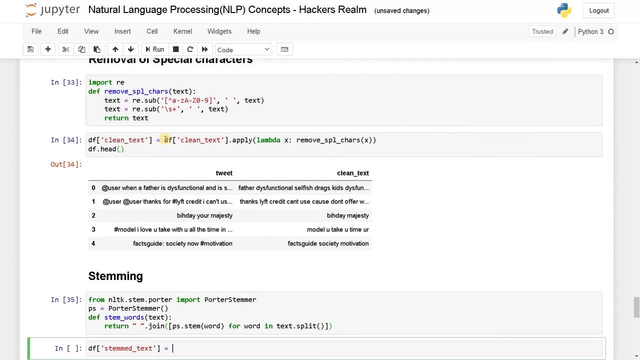 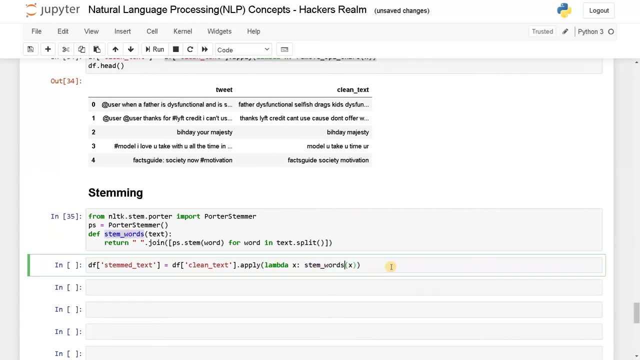 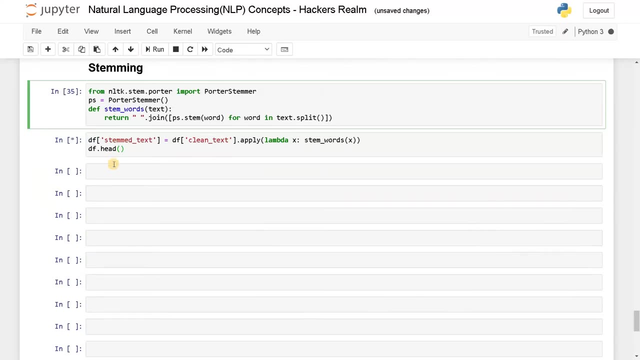 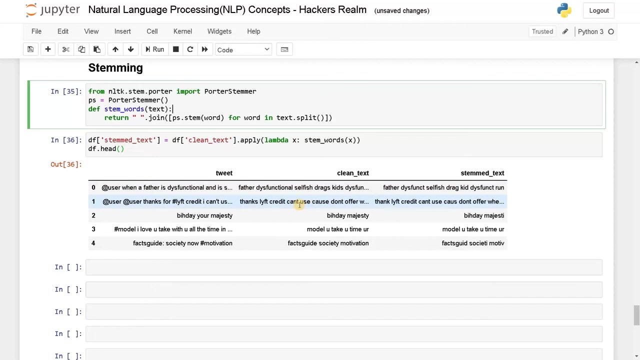 text equals. we'll just use the same lambda function to call this, that is, stem words. okay, now let's run this, so this will take some time. yeah, now it's done. we can able to see some of the words are like truncated from the clean text here: thanks is uh truncated to thank uh. cause is truncated to c, a, u, s without a, e and uh. 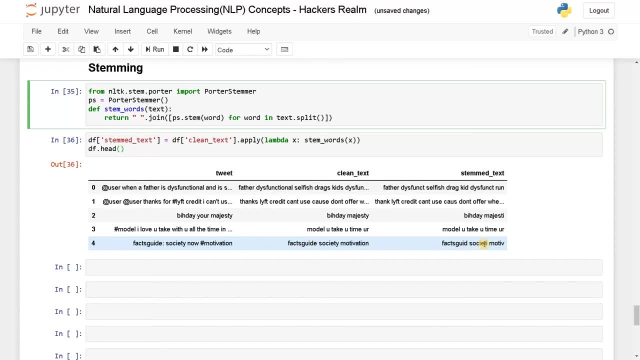 what other things are truncated here. fax guide is like truncated to like uh without a e, and society is also like converted to society with uh instead of y. it's just having i. motivation is just converted to motive, like that. we just find the root word and this is how stemming works. now let's see about lemmatization. 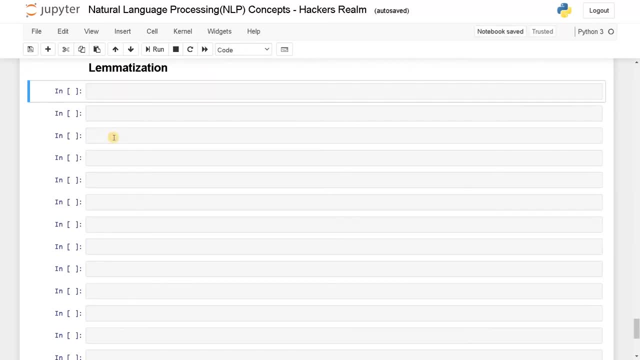 lemmatization. so for lemmatization, uh, it's actually uh better to do with the po's tagging. we already seen all these concepts. you can also check with the post tagging. we already seen all these concepts. you can also check. you can click on the right top corner if you want to check out the playlist for. 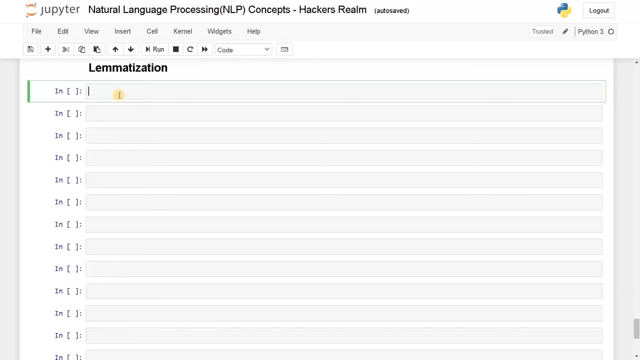 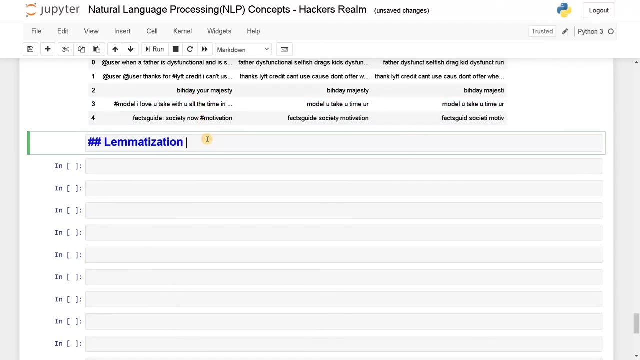 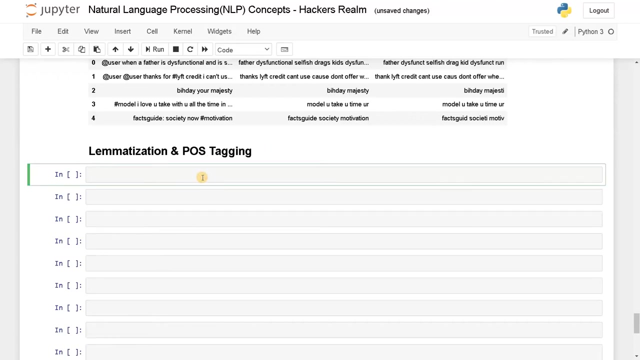 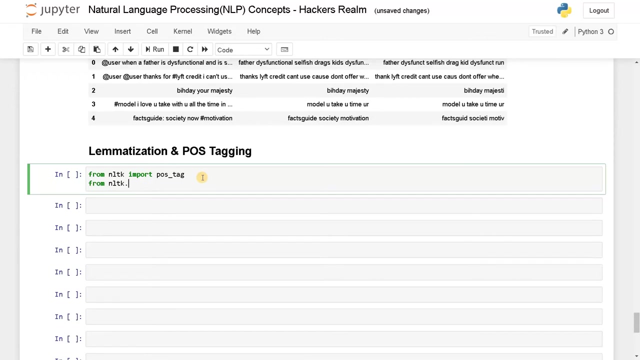 a detailed explanation of these concepts. for this i'm going to combine both lemmatization and paths of switch, lemmatization and pos tagging. okay, now i'm gonna import both of these from nltk import pos tag and from nltkcorpus corpus import wordnet. 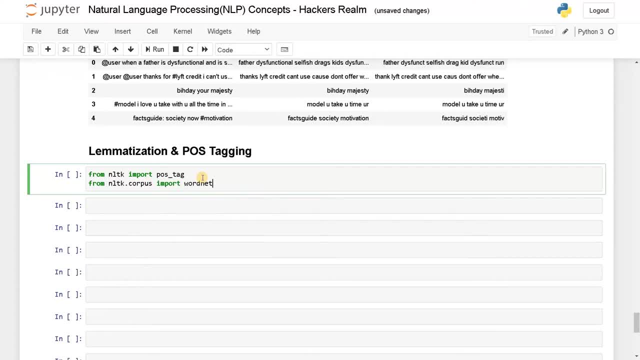 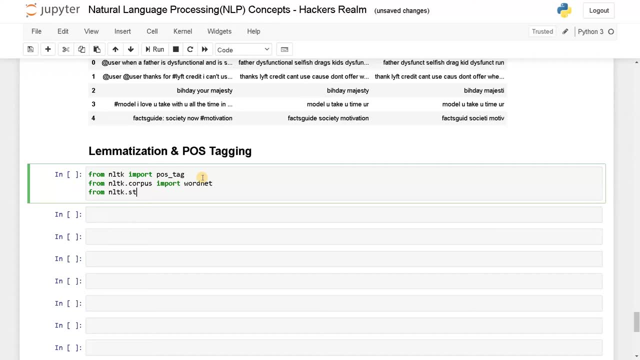 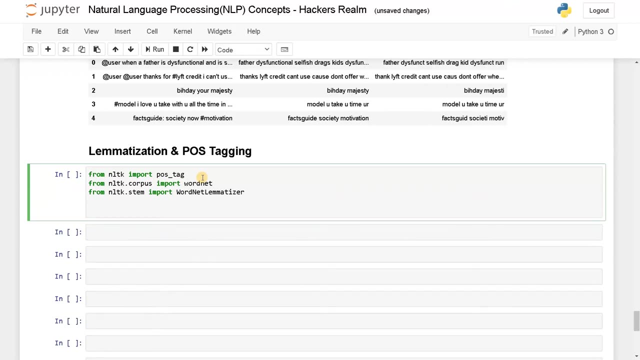 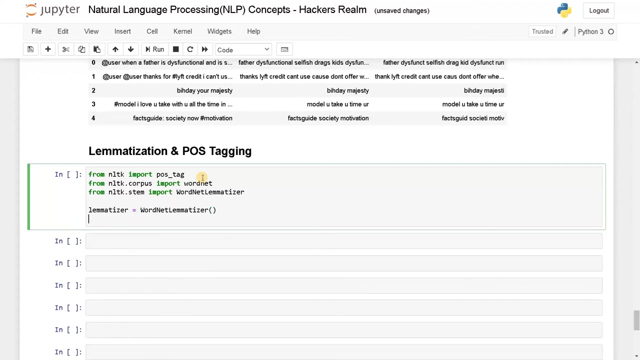 wordnet and for stemming: wordnet nltkstem. import wordnet lemmatizer. okay, these are the modules we have to import and we will initialize. the lemmatizer equals wordnet lemmatizer. initialization has been done. and uh, for the pos tagging, we'll be getting like. 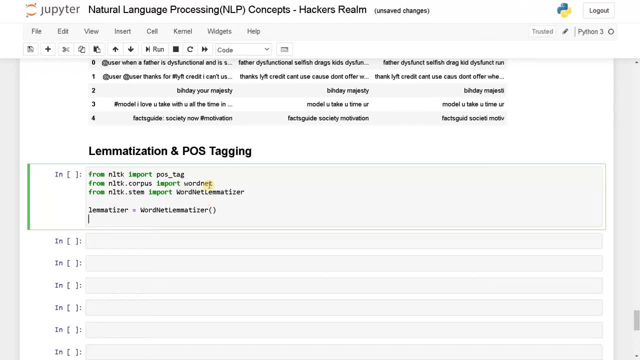 different pos tags, like nn, that represents noun, and even in the noun they have like multiple things. so we will just map that. so i'll say word net map. i'll just create a dictionary with n equals word, net dot noun. you can also see how it looks like. 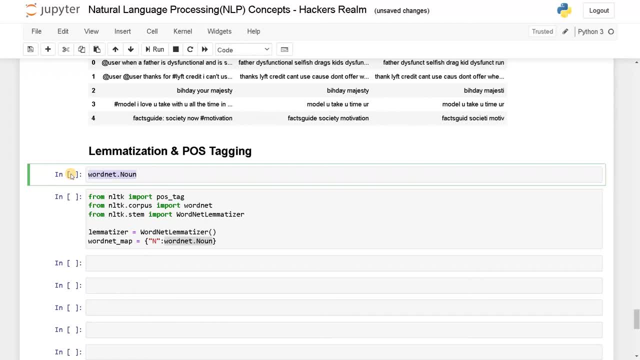 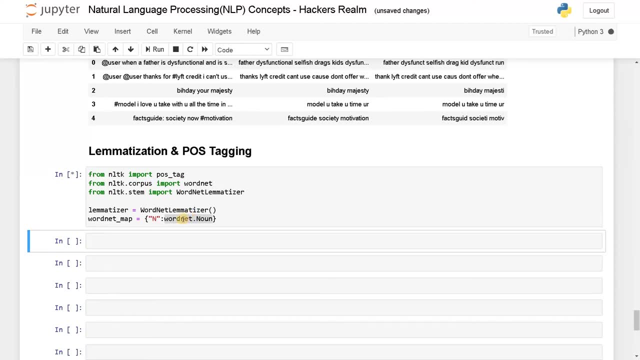 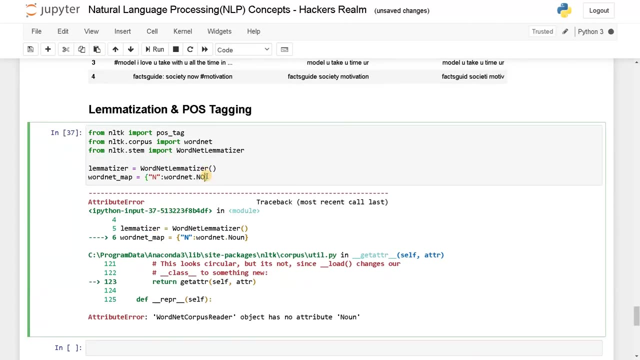 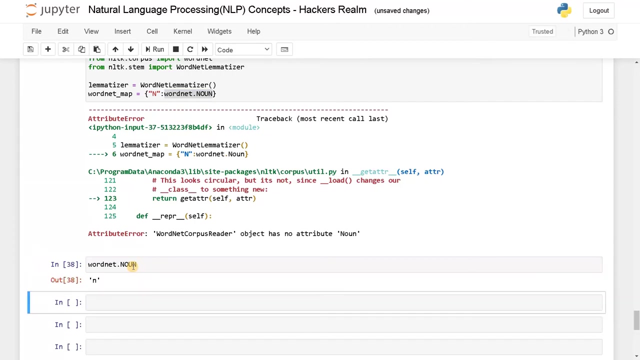 okay, i have to run this once at least. okay, let me just run this once. okay, this is like a capital noun. let's take this out and run this separately. see, it's just converting into like a smaller case. so these are the cases that will work when you are using a lemmatizer. that's why i'm just 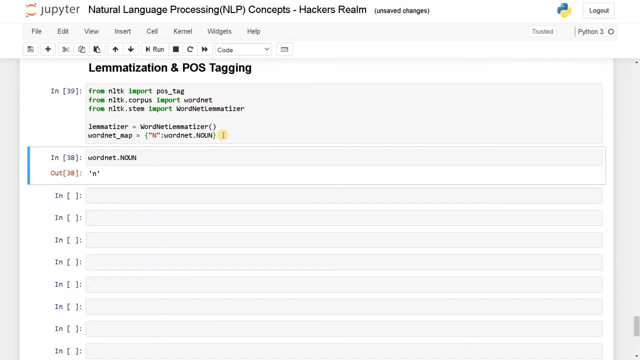 creating a dictionary. let's just run this once. okay, now i'll just do this for the verbs and other words as well. so v, that will be word net dot verb, suggesting very slowly, i guess, and after that i just have j, word net dot adjective and finally we have r, i'll just say word net dot adverb. 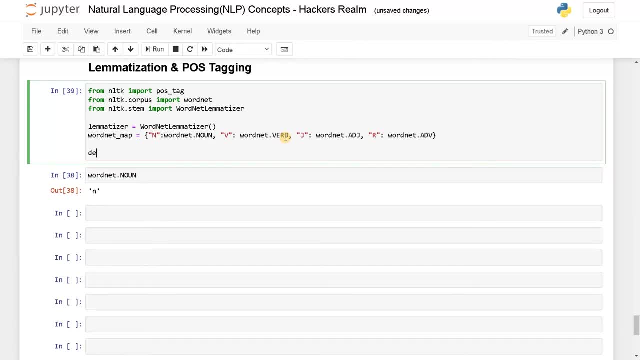 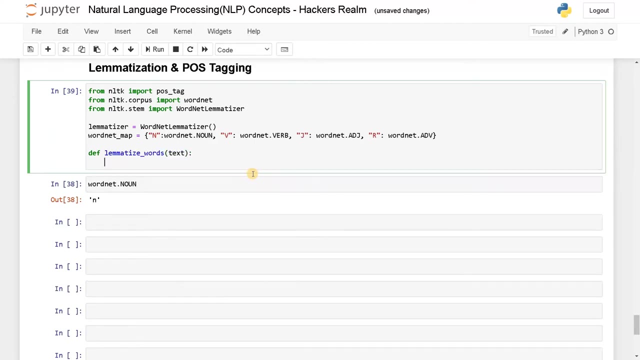 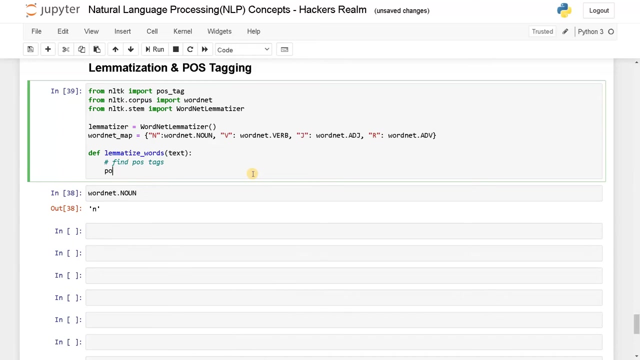 okay, these are the mapping. uh, we have to do and finally, we will uh create a function. before that, we have created stem words here. i'll just call it as lemmatize words- lemmatize words of text. okay, here we go here. First we have to find POS tags. I'll just say: POS text equals POS tag of text, dot. 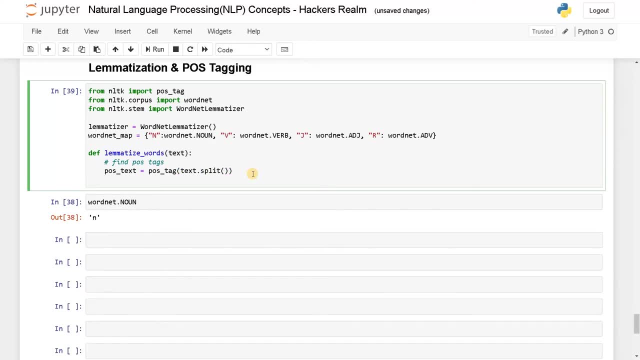 split. Okay, after finding the POS tags, we will just use the return statement: dot. join in a list called the lemmatizer, lemmatizer, dot lemmatize, lemmatize of. pass the word as a parameter And after that we will get it from the word net map, So word net map Here. 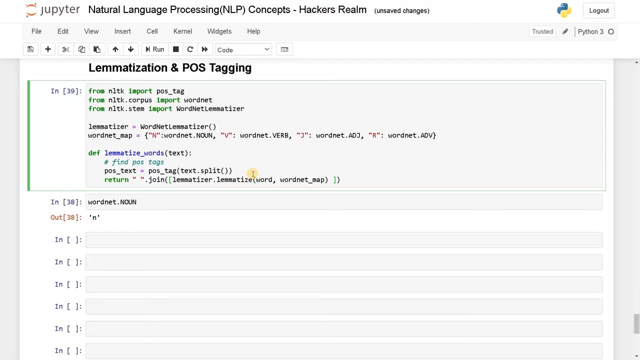 you can just get it from the dictionary. Before that we will just iterate through that POS tag text, that is POS text for word, comma, POS in POS text. So now we have two things, that is the word and POS tag, And here we will just use dot get function. What it does is: 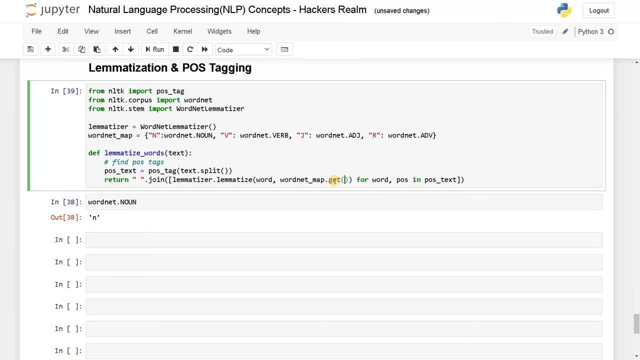 if the key is not present means it will also suggest a default value. So here I'll just take the first character. POS is POS, it is a parts of speech, And with zero I'll just take the first character. Okay, I think okay, if this particular character is present. it. 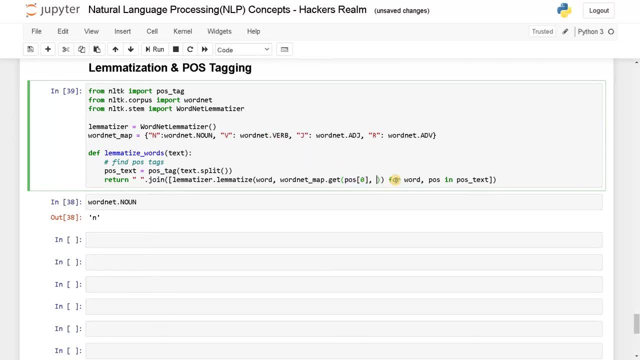 will return it from the dictionary If it is not present. means we will by default have word net dot noun. That means other than these four. if you have some other POS tag you got, means we will just pass it as a noun. 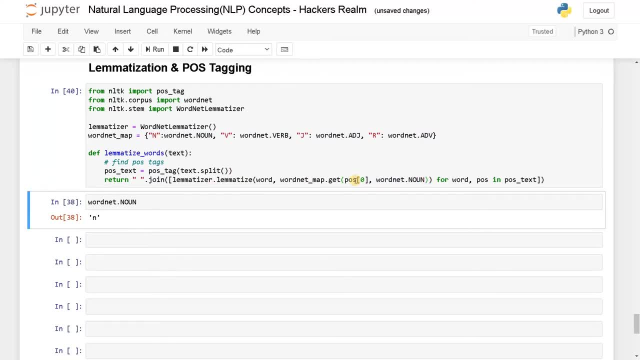 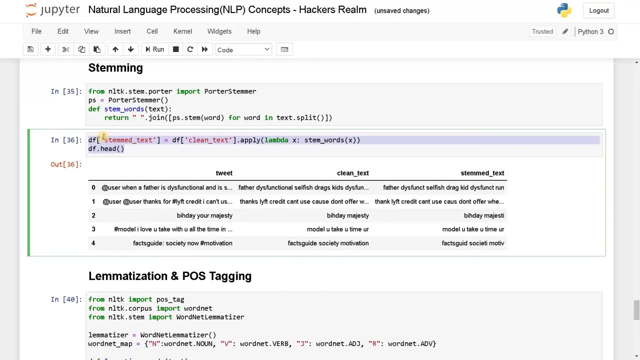 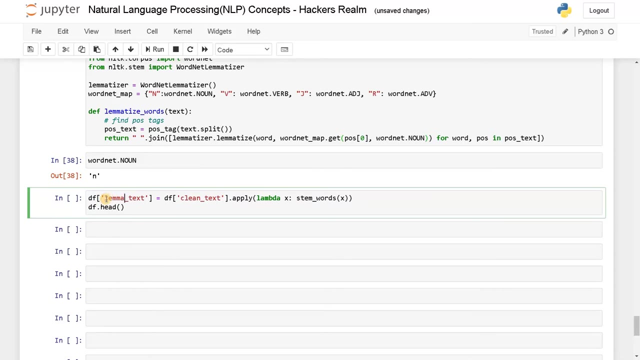 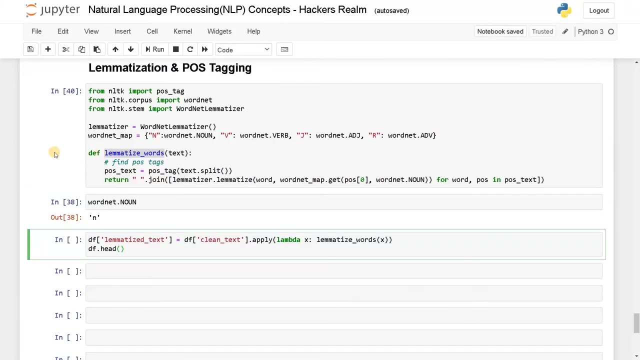 So it will be easier for us. Now let's run this again. let's call the function, and here, instead of stem text, I'm also gonna create like lemmatized text, lemmatized text, and here just pass lemmatized words. run this. 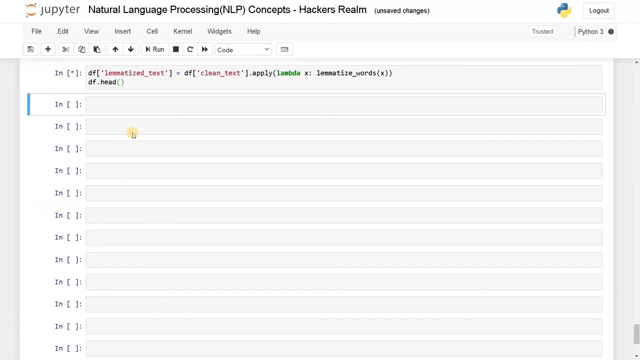 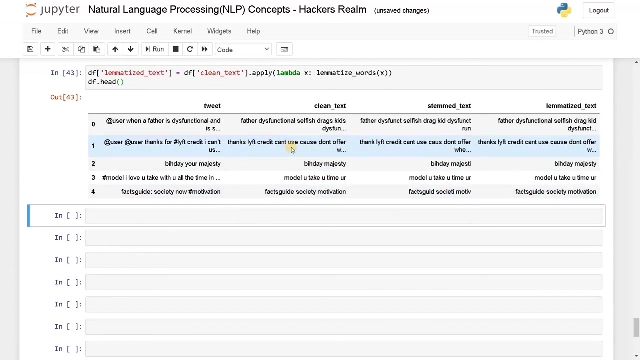 and this. this could take some time because this will take some more processing compared to the stemming. Let's wait for some time. Okay, Now that's pretty much done. Let's see whether it's truncated or anything Here. it just converted this kids to kid. 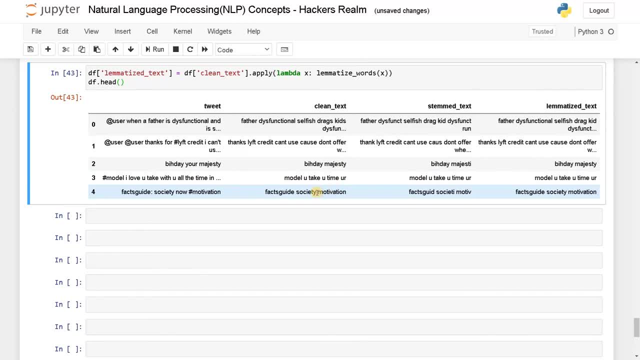 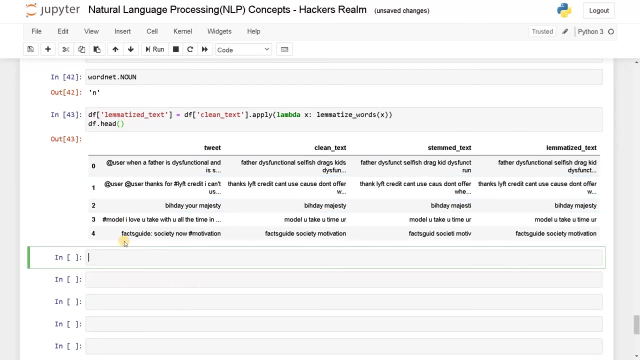 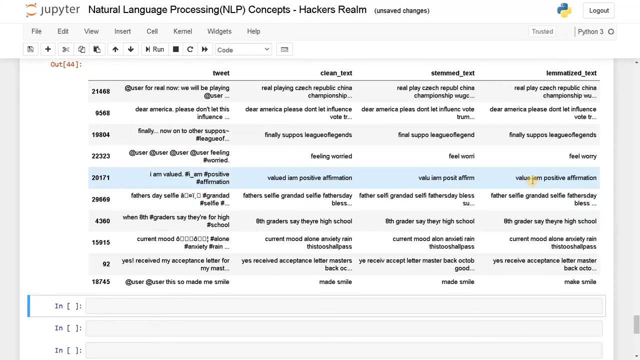 What other conversion has been done? Think I can't find any in this clean text. Should I shuffle and see? Okay, Maybe that would help, So I'll just use shuffling and see the top 10.. Okay, Let's see from valued. it just converted to value. 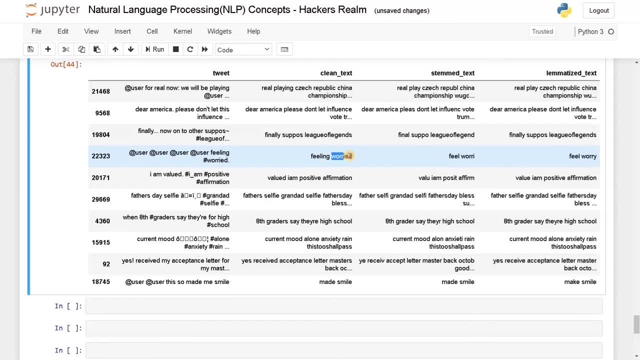 Here feeling is converted to feel. worried has been converted to worry. So you can clearly see the difference here also. It just converted to feel But worry. the letter wording is different, So this characters won't be present in the dictionary, But here in the lemmatization it converted into a root word that will be in the dictionary. 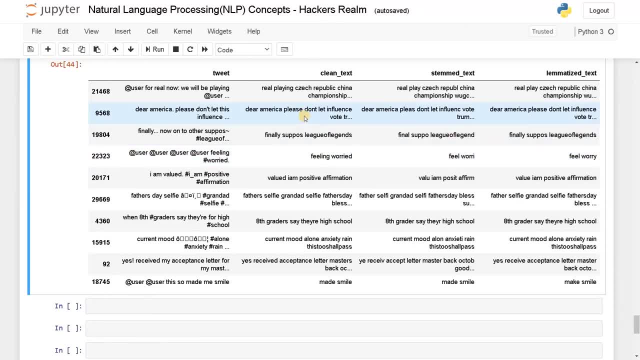 So I think this is like much better. So it depends on the use case. You can use either stemmed text or lemmatized text, but most of the time I just prefer lemmatized text. So these words will be present in the dictionary. 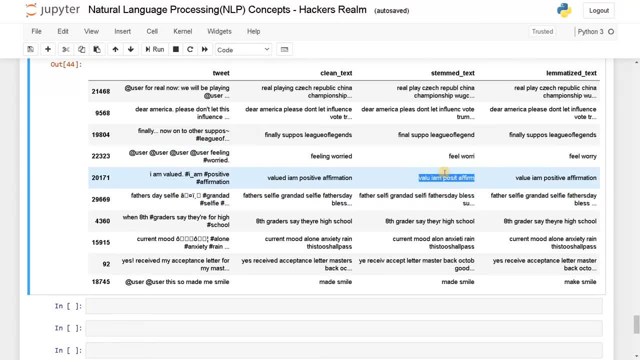 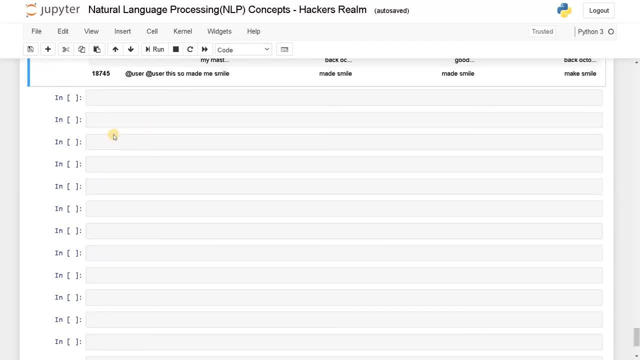 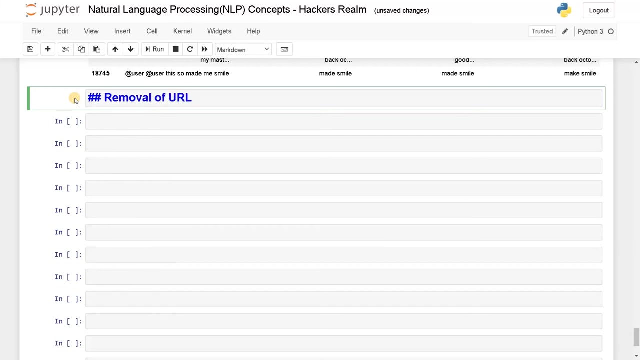 So it will be easier to understand compared to stemmed text. Now, that's done. Apart from that, I'll just teach you like a few additional tricks, if it is like useful, if you have the data set. So the next one is removal of URLs. removal of URLs because most of the time we don't 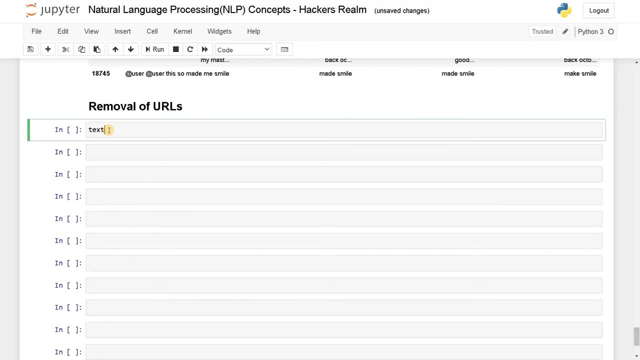 need the URL. Okay, So let's just create a text here: http//wwwhackersrealmnet. So this is the URL of this channel. You can check. it is the URL of the channel hackers realm, But in some of the data set you don't need this URL actually. 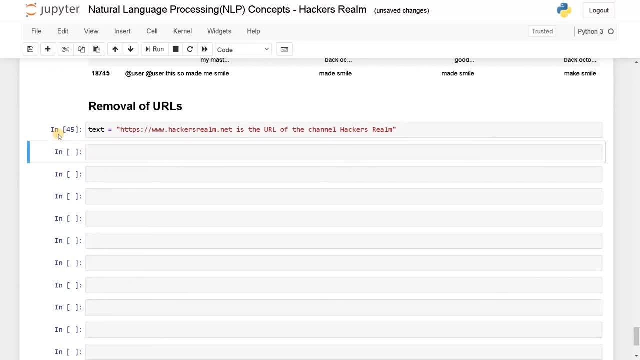 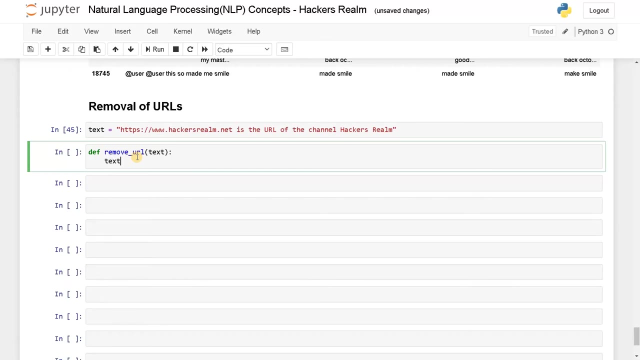 So you want to remove it? We will just see how to remove this Now. I'll just create a function def- remove URL of text. Here I'll just use regular expression itself, So text equals, or I'll just return resub of the pattern. 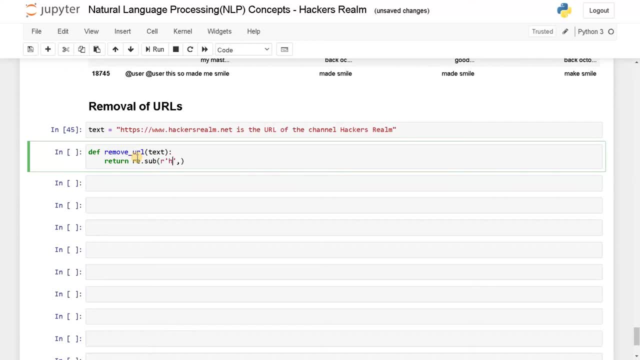 So that the pattern will be like this: Okay, Do not use long bracket on your style. So click on a dot- welco- and say if after this we will be having that www handle. So if you just had the dot in, sometimes it will just consider the regular expression. 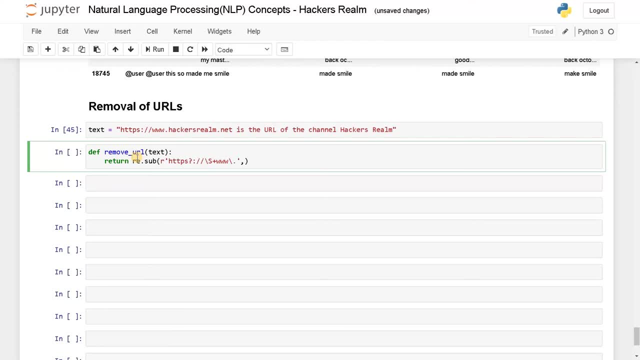 symbol. so that's why you have to specify, if you want to specify any symbols, and after that you can have like any number of words. so that will be backslash capital s plus. i'll just replace it with like empty string. it'll just remove the whole thing and i'll just pass the text. so this: 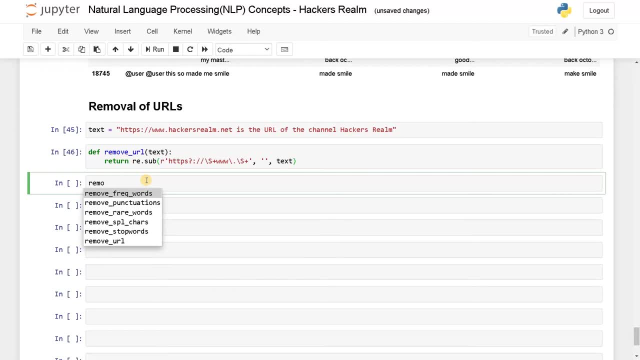 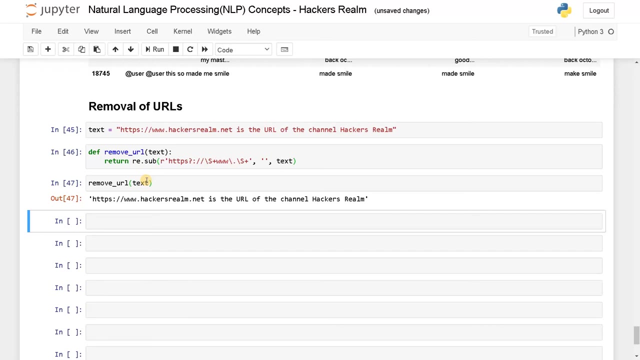 is the function. let's check it whether it's working or not. remove text. sorry, remove url of text. run this. it didn't work. okay, i just missed one thing here. i just have that r symbol. run this. run this. yeah, now you can clearly see the entire url has been, uh, removed. you can also check it. 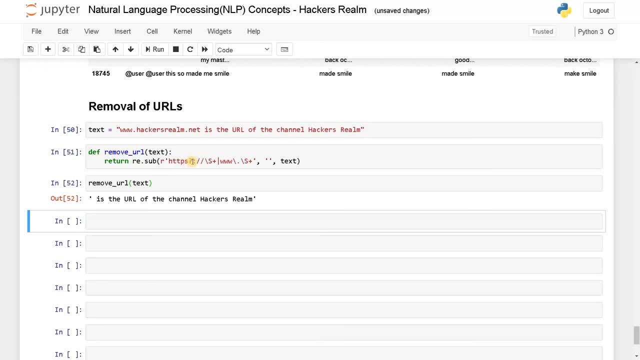 like this also see, uh, it either considers this https slash slash or this whole wwwhackersrealmnet. so any of the format will work. so it will find any of the url and remove it, so it will be helpful in this case. so this is removal of urls. 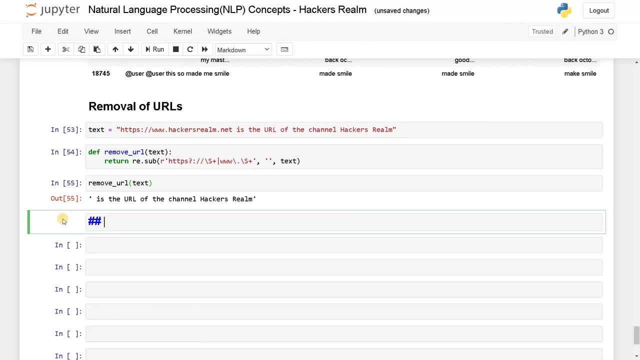 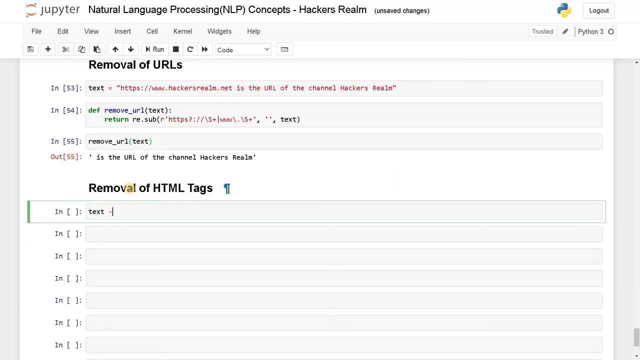 now, sometimes you also have like a html tags in your whole data set. you just want to get that particular text from the html. so for that we'll just remove removal of html tags. remove html tags again. i'll just create a text with some tags. i'll start with html, slash html. inside you will have body, body. 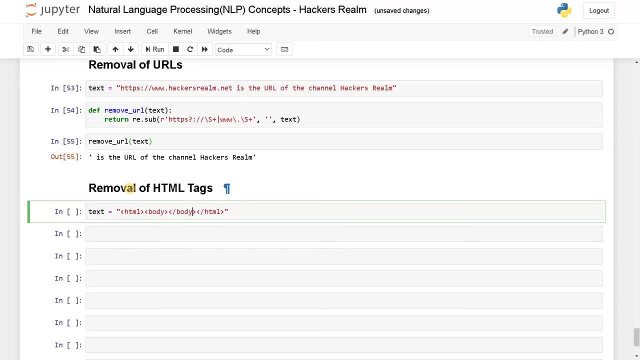 body and for that just have some space. so in between I will have a paragraph tag, paragraph tag. so I just have this NLP text: pre-processing tutorial and close the tags. and what other tag you can have? maybe I'll just have a h1 tag, that is. 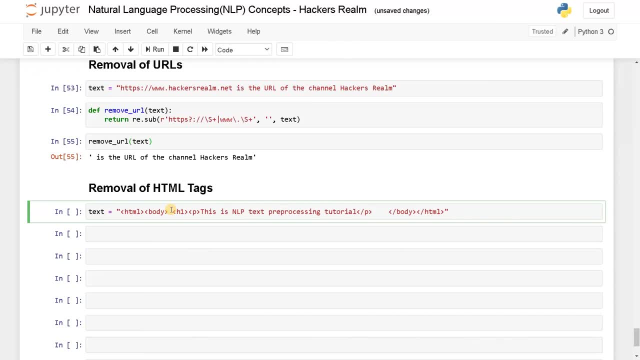 also, like commonly there, I'll just choose hackers realm and close the h1 tag, slash h1. so that's it. you just want to get that important text with a this HTML tags. let's run this now. again, we are going to use the rejects in order. 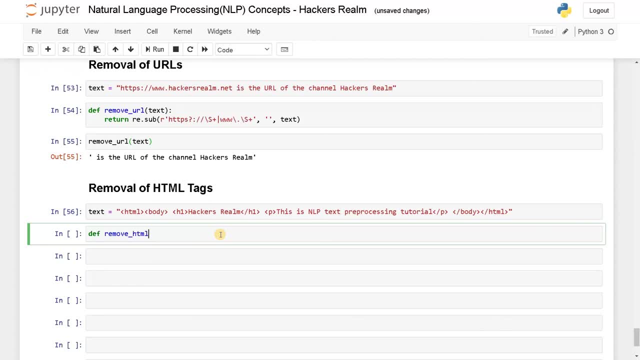 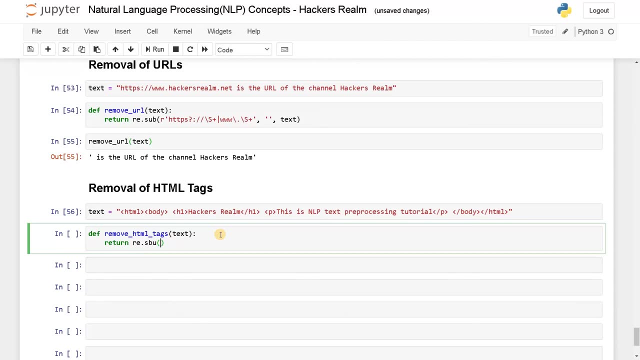 to remove this. so remove HTML tags of text now written. read out sub sub of regular expression of opening tag: closing tag: you inside it dot, star, question mark, so whatever, like. if you have this format like, it will just remove the whole tag. so this is like one or more characters. 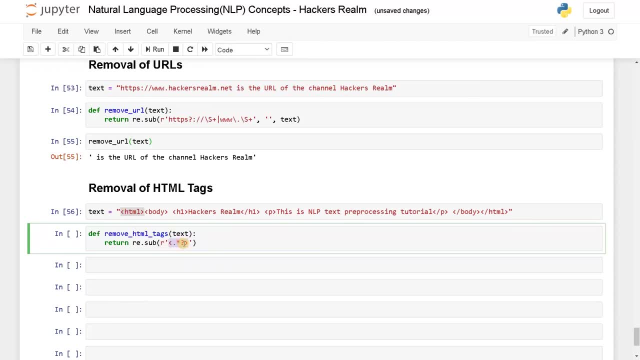 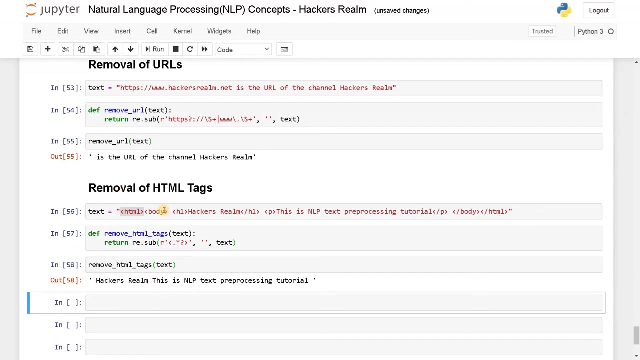 present in the particular pattern. so this will just remove the HTML tags for you. I'm just gonna replace it with like empty string. pass the text, remove the HTML tag. it COLOR. now let's remove the HTML tags. remove the HTML tags of text and this. now you can clearly see. we just remove all the HTML tags. 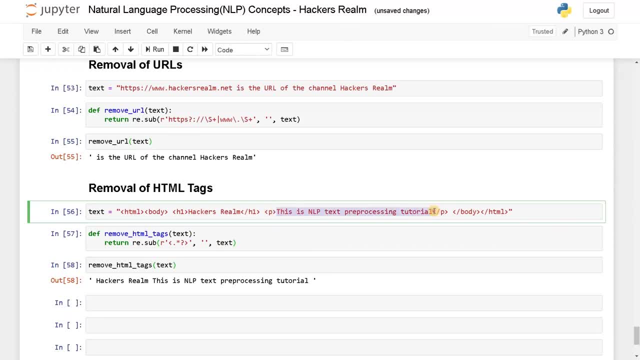 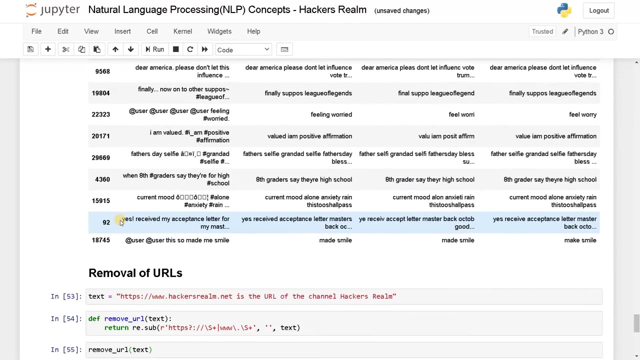 we are just getting one lead, this important text that is present in the tags. so this is how you can easily remove the HTML tags from the text. if it is present. you just have to call the function like this, like apply X, remove HTML tags, so it will just remove HTML tags in the whole data set and I think we have reached the 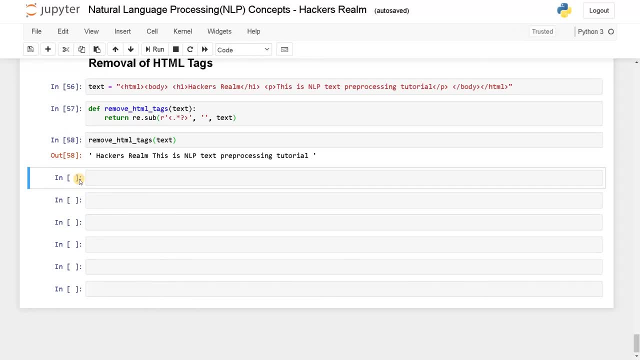 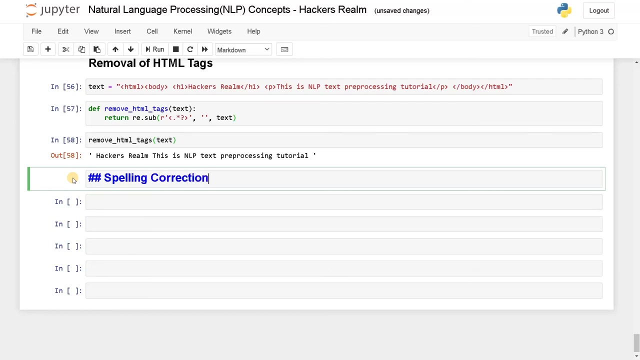 final part, that is, spelling correction. sometimes the person who are like creating the data, or if you are getting the data from the internet, means sometimes there will be a mistake of words. the spelling mistakes will be there so you can easily correct the spelling. so spelling correction. so here. 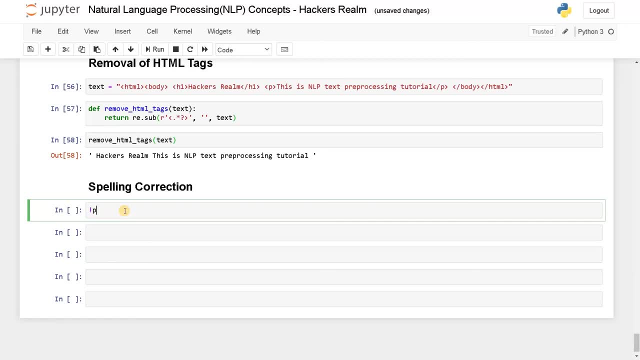 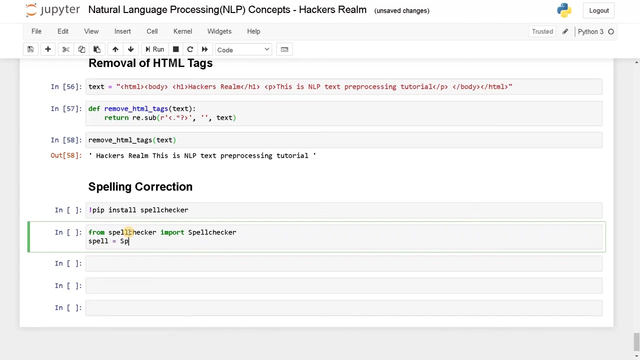 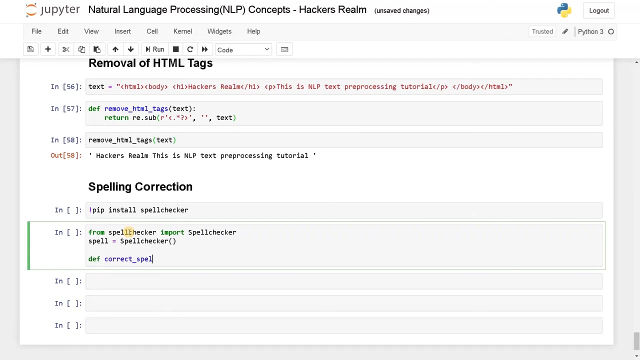 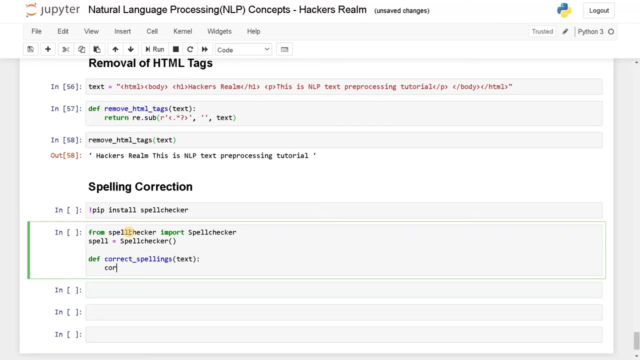 for this you have to install a module, so that will be pip. install spell checker. so I already installed it, so I don't have to install again now from spell checker. import spell checker and initialize it. spell equals spell checker. now create a function: correct spellings of text. so first I'm just gonna get like the corrected text: equals. 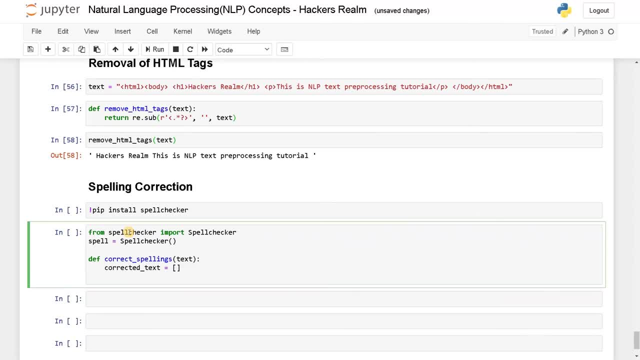 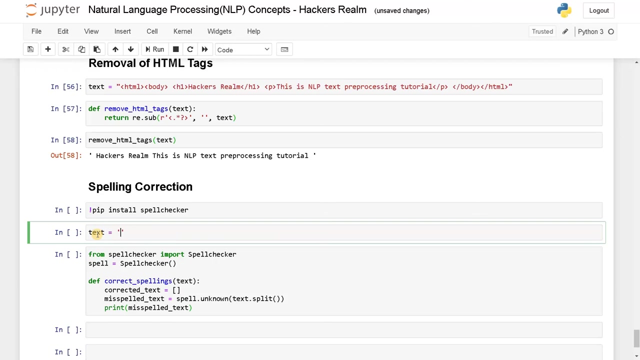 this and I'm gonna get only the misspelled text first. so misspelled Neighbor eats. most spell text dots split, so this will contain all the misspelled text and also print this one's to see what is inside it and our also create a text for us: Nature is a beauty. So this is the text I'm going to go with. 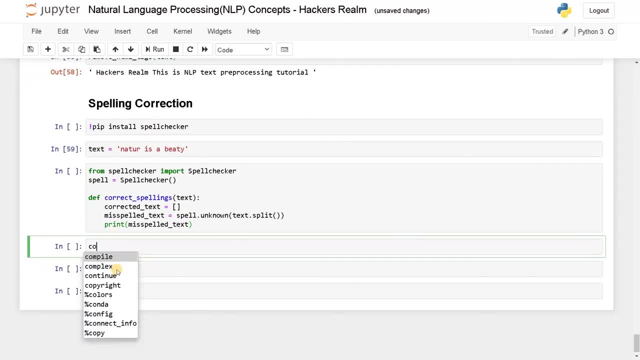 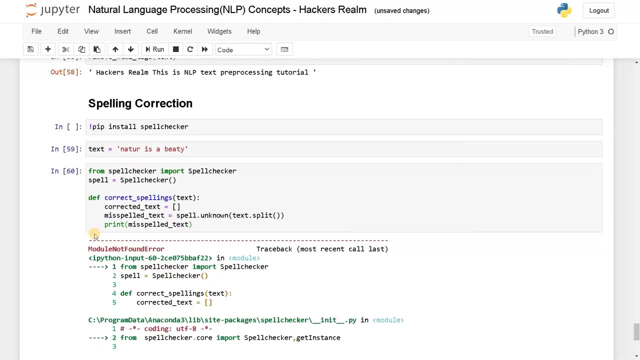 And here I'm going to call the function: correct spellings. Okay, it's not even run. Okay, some module has been missing. Most of the time it will just install all the module, but this time some module has been missing, Okay. so here, instead of using spell checker, use 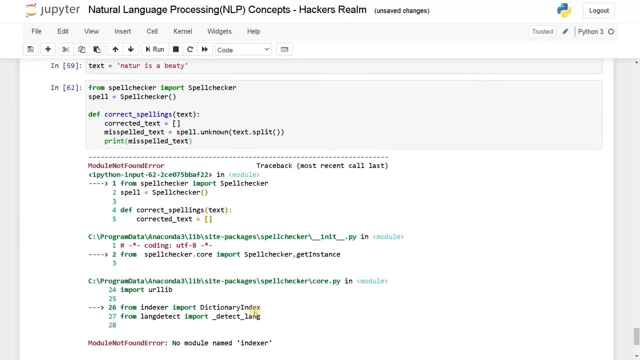 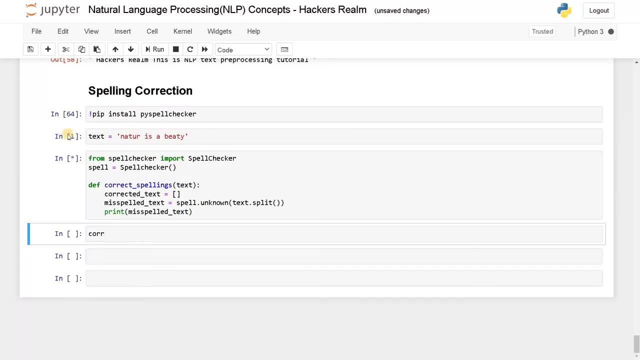 PI spell checker, because I in that module, I am facing this indexer error. Now, let's run this again. Let's rerun this. Okay, this is spell checker. Okay, now it's working. Let's call the functions: correct spellings of the text So you can see the unknown words. 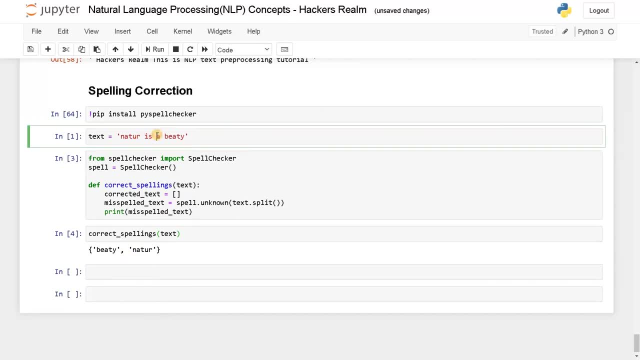 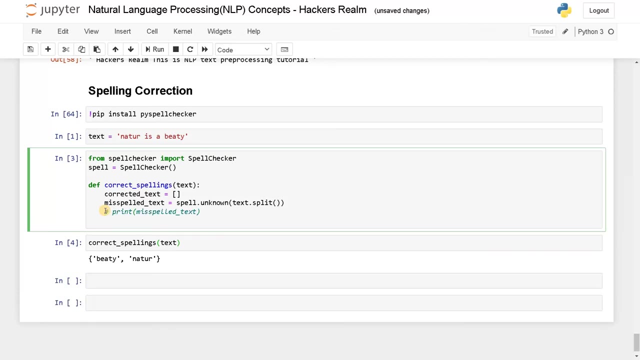 Here it's just a remote. I ignore, this is an A, So these are the mistake, mistaken words. So it just taken it in the misspelled text. So I'll just comment this. Okay, after that you have to go word by word. So for word in text: dot split. 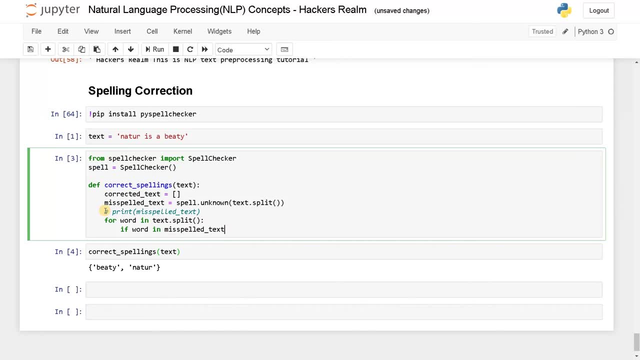 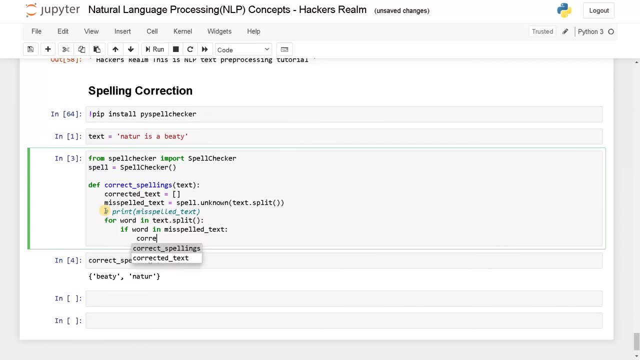 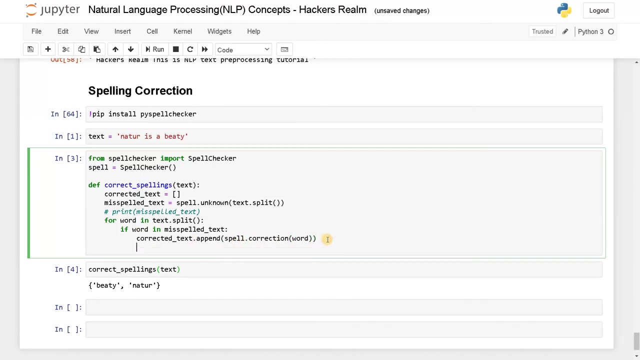 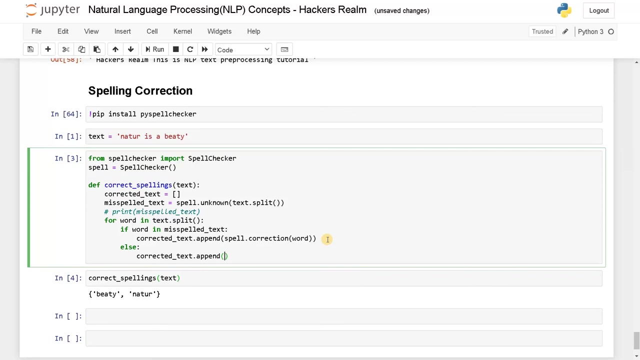 If word in misspelled text, then corrected. corrected text: dot. append of spell, dot. correction of the particular word. So here with this will be just doing the correction and appending into the corrected text, Else we'll just directly append the word dot. append the word. 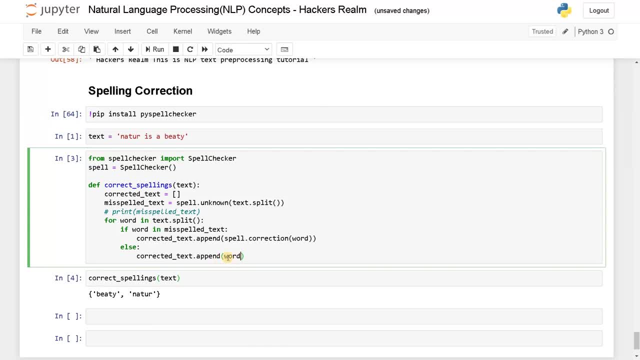 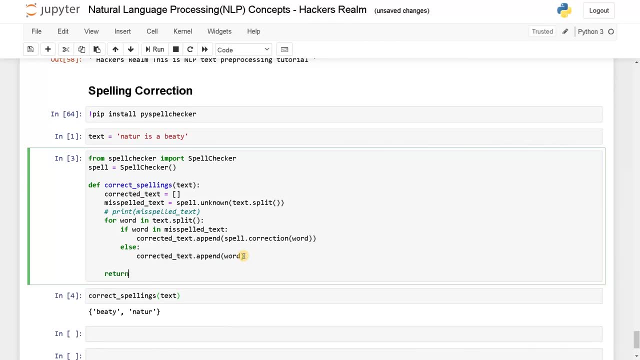 So if it is not in the misspelled means, we don't need to call any function, we'll just directly upon the word that is, this is and ye, Okay, after doing this, we have to return the text. So written space, dot, join of corrected text. run this, run this. So here I just converted Nature. 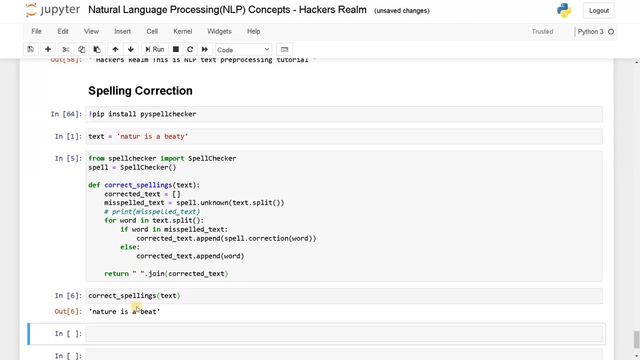 is a beat. Okay, that is also like another word instead of beauty, it's just gone for a Beat. Let's say with this word What is showing? okay. so if i just treated it differently, it's just correcting the word what i'm like. 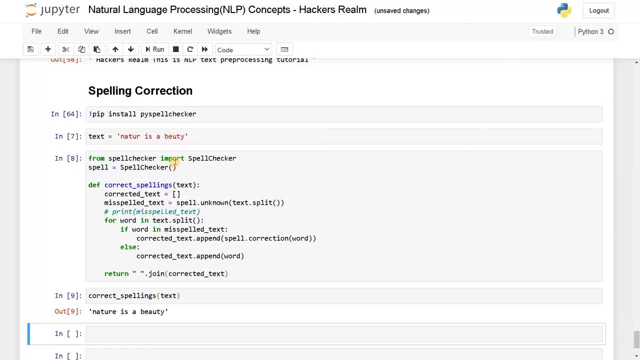 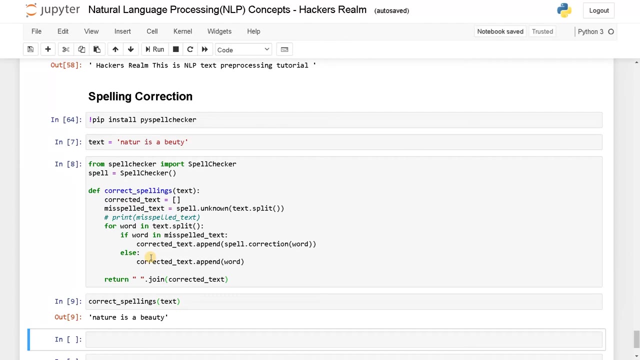 intended. so beat means it is also like a word that is present in the dictionary. i just converting the spellings, so that is also like feasible. this is how you can able to correct the spellings in the data set, so this will be very helpful in order to clean and enrich the data you already 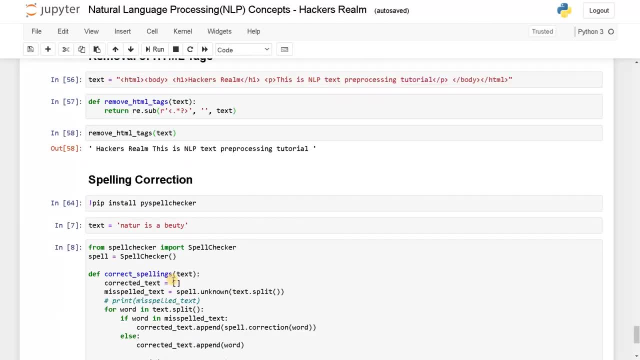 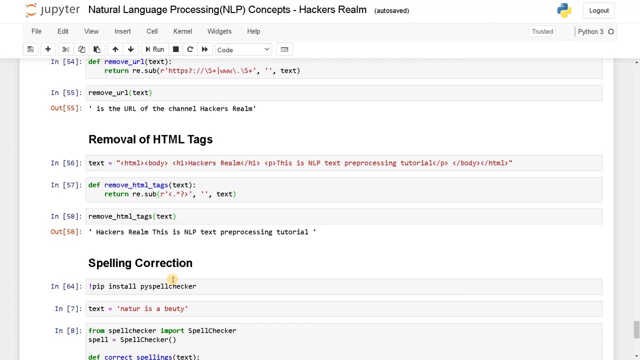 have- and i think that's pretty much it, guys. we have seen like various techniques for pre-processing of text and you can also see some of the other pre-processing steps in the previous videos, like tokenization, part of speech, tagging. you can also use it as a features, like